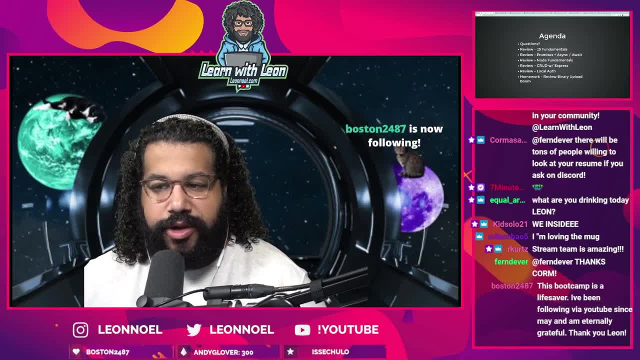 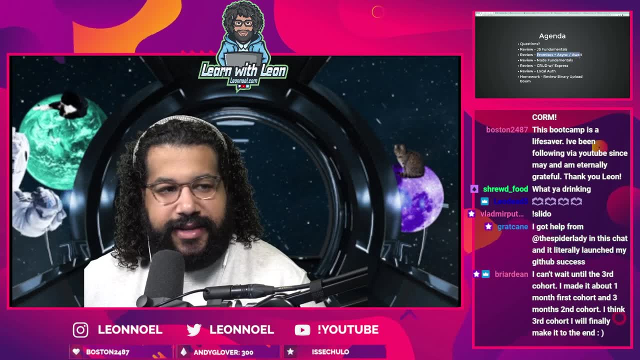 let's get into it. let's do a little. let me walk you through what we're going to do today. so we're gonna start off with js fundamentals. right, we're gonna start off with js fundamentals. uh, we're gonna go over promises: async await. we're gonna go over node fundamentals. we're. 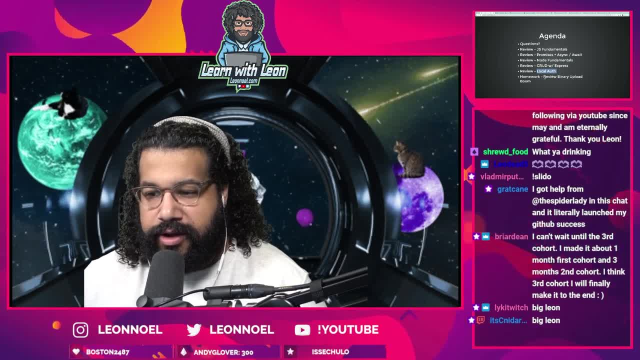 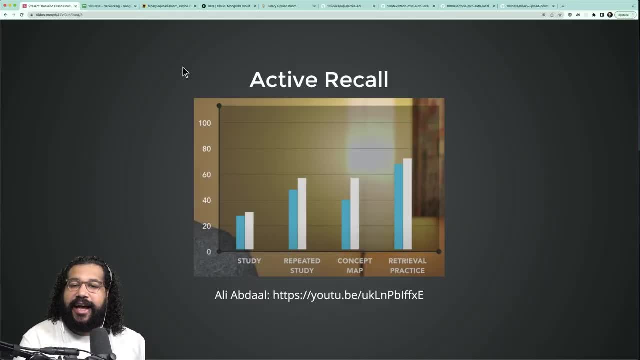 gonna go over crud with express, we're gonna go over local off, we're gonna review our binary upload, boom, right. and so if sit through these six hours, right, if you sit through these six hours and you don't do any active recall, it was a waste. right, it was a waste, we know. we know that. 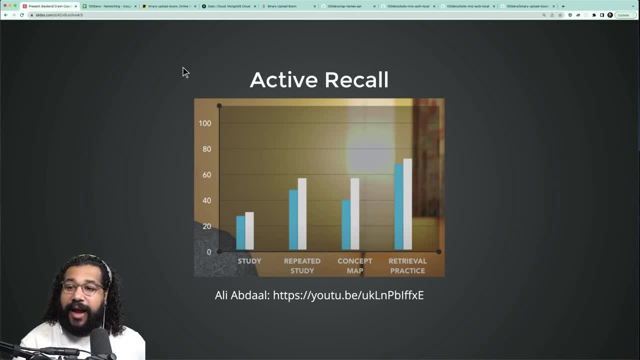 there are specific study habits that will literally change the game and what you're able to retain and what you're able to use going forward. software engineering is a cumulative career, the way that i go through lectures, because i'm always learning something new, literally always something like. 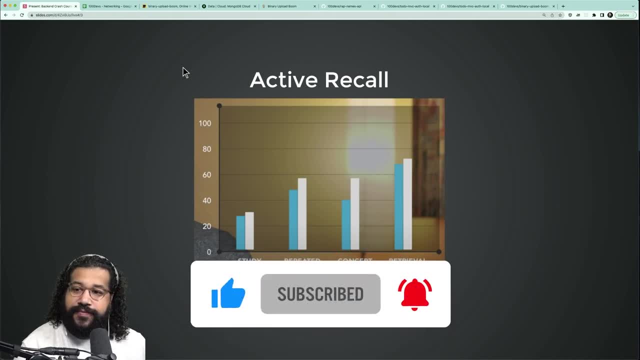 one of my favorite things to do is learn something new, and when i am learning something new, active recall is a key part of my process. the way that i go through lectures right or through somebody trying to teach me something is: i don't take notes. notes don't work, um, i take questions instead. so, as 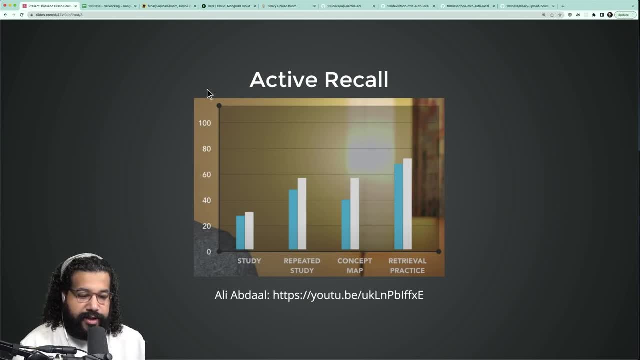 i'm going through and somebody says, um, let's say. somebody says, uh, html is the content of your website. i would say: what language makes up the content of a website? so that's the question i would write down. so, instead of taking notes, i'm taking questions at the end, right at the end of my 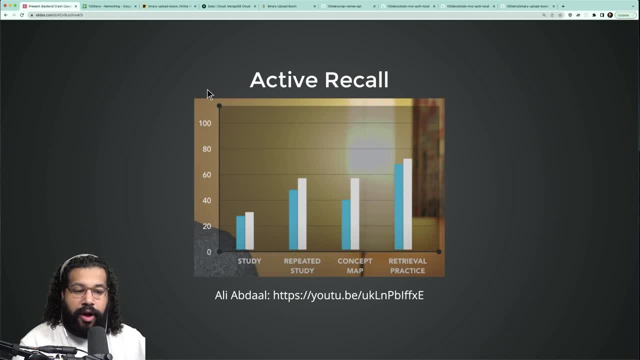 lecture or video, whatever the heck i'm watching. i go through all those questions and that's my active recall. that's my ability to recall all the things that i just learned. now. there was a study, and ali abdul has a wonderful video on this- this. 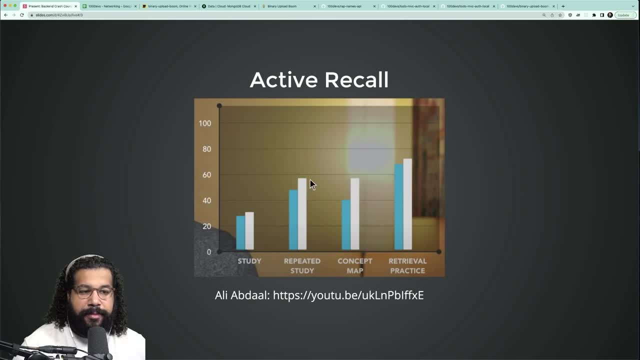 is their their graphic here, where they looked at a group of people that re-read a chapter four times. so this is the group of folks rereading a chapter four times, and this is the group that read the chapter once and then recalled to themselves the thing that they just learned. 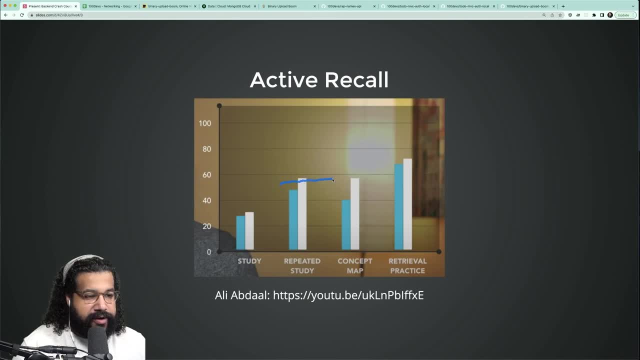 what this broke my brain. i know if you've been around here, you've seen this a bazillion times, but this, this literally broke me right, because i was the type of person that would reread multiple times, that would thug it out like i was going to put in the work and hopefully get there. but these people 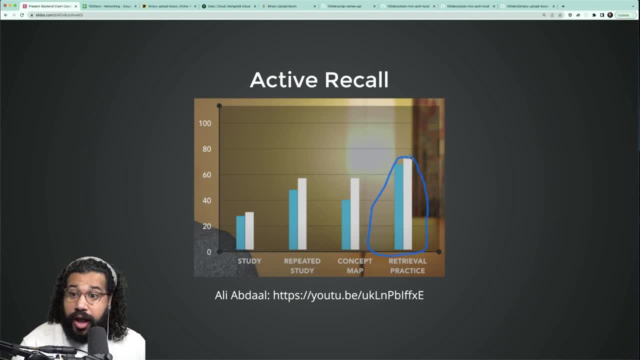 are doing a quarter. a quarter of the work and doing better than people that reread it four times. think about that. a quarter of the work and getting better results. so make sure you're incorporating active recall. for a lot of folks, uh, they'll active recall at. 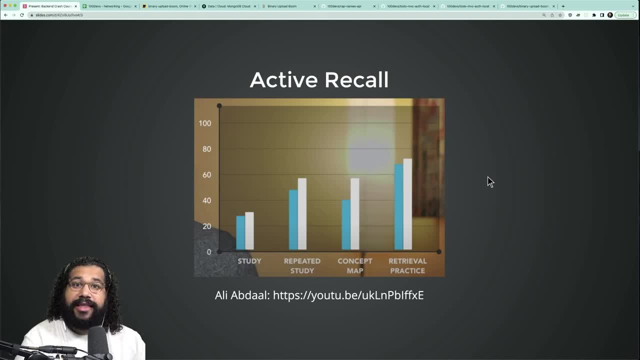 the end of each chapter. i like to active recall after every couple of paragraphs. my brain teleports when i read, right, my brain teleports when i read, and so i like to actively recall after each chapter- yeah, that's right- after each couple paragraphs, what did i just read, what did i just do? 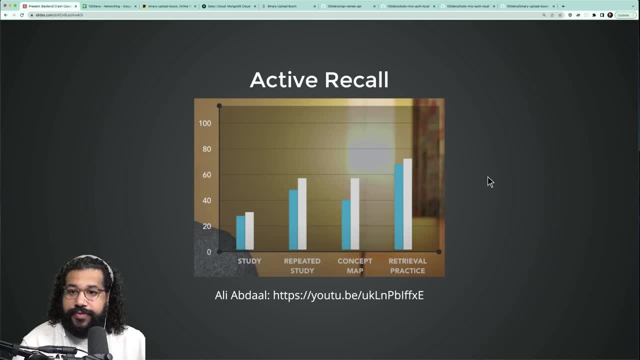 now what do i do after i do it again? right and so um super important practice: if you're not doing it, even if you've been with us the whole time, you're not doing it. start doing it now. literally put in a fourth of the work and get. 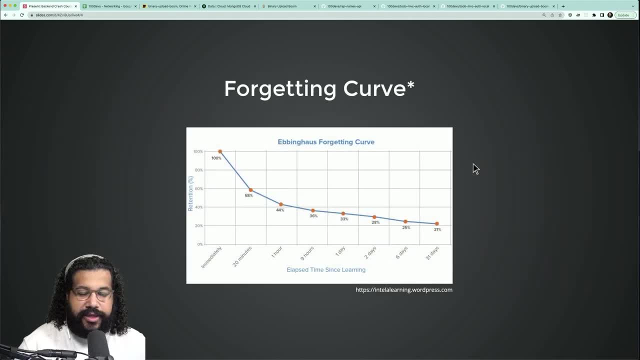 better results now. the other important thing to keep in mind is that we forget stuff. right, we forget stuff, we will. we will sorry one second, we will learn something, and then by the end of a month, there's an 80 chance that we have forgotten what we just learned. let's think about that. sovereign during is a 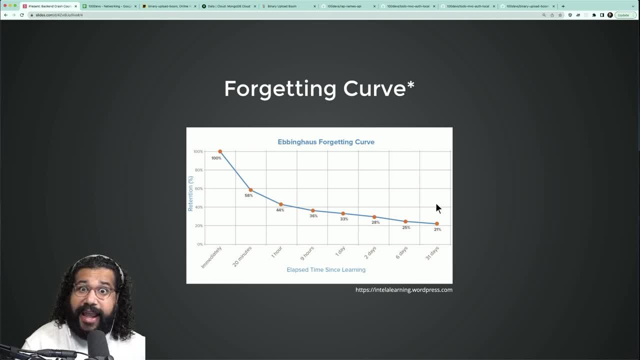 cumulative career and there's an 80 chance that we forget the stuff that we just learned that month right, and so we can't let that happen. you can't put in all this work and then be in an interview and they ask you to use some css and you can't do it right, or they ask you to do a certain coding. 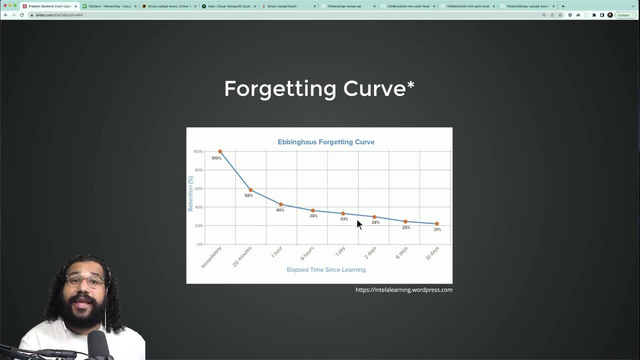 challenge that you know you've already solved. that's the worst. that's the worst. that's the worst. the worst is being in an interview. they ask you a coding challenge that you already solved and you can't remember how to do it right, and so we can flatten our forgetting curve. 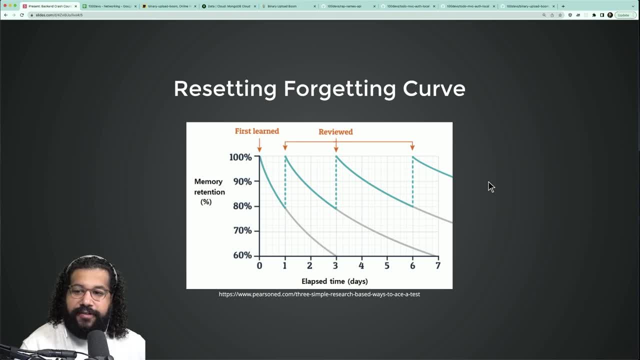 right. we can flatten our forgetting curve right and make sure that we do not forget stuff for the long haul, and so what we can do is we can review material over and over again, and each time we review the material, the length of time that it takes us to forget. 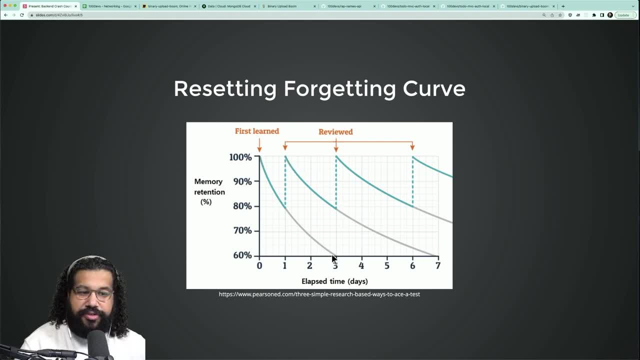 increases. so the first time you learn something, by the end of three days there's like a 40 chance that you've forgotten it right. and then the second time you review it, it takes like seven days for there to be a 40 chance. and you keep reviewing and it keeps flattening and flattening. 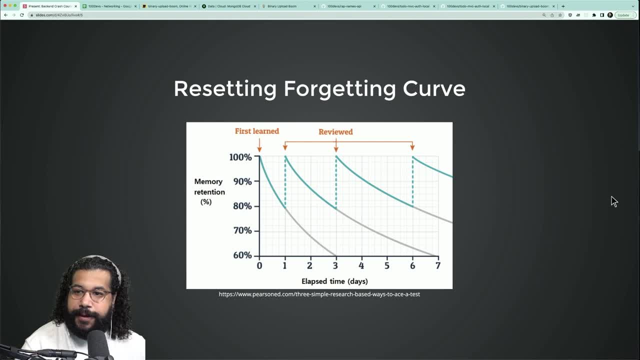 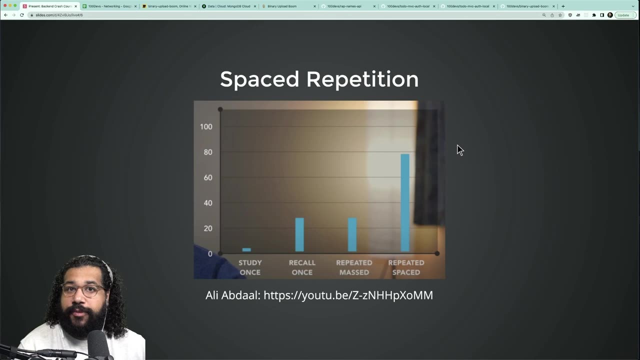 and flattening. right, right, all right, he's flattening and flattening and flattening. so the more you do your resetting of your forgetting curve, the more likely you are to remember, and this is called spaced repetition, the tool that we mostly, mostly use around these parts, or the tool 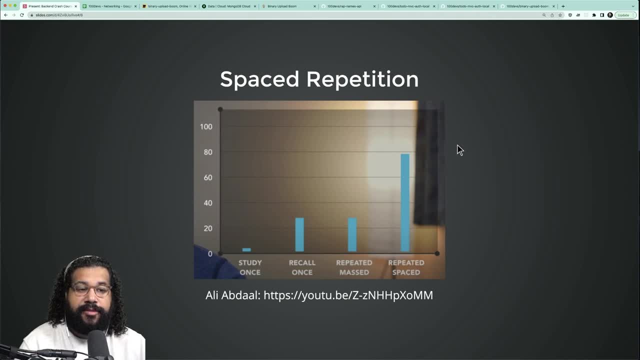 we do use around these parts is called anki- or anki, if you're hermione right- and this tool is flash cards with an algorithm behind them, and when you use this spaced repetition tool, it serves up the material that you need to see. so you don't. 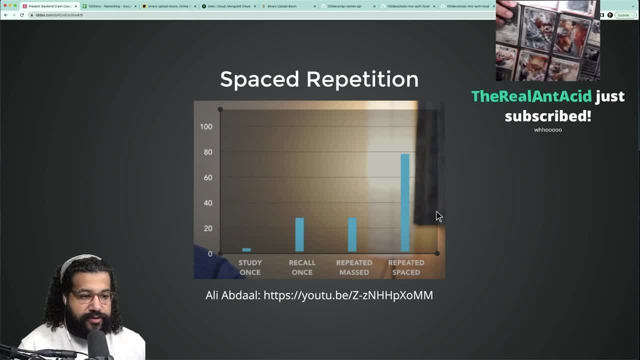 forget what's happening, and so here is something that's really interesting. here's someone that spends a saturday, right. that spends a saturday studying something over and over, right. so you, you reread something a couple of times. you, you have your flash cards and you spend, you spend a couple. 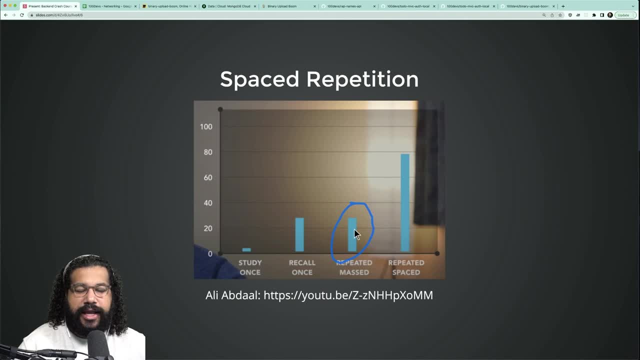 hours on saturday going through your flash cards, right? so let's say you have five hours a week, right? some folks will take their five hours. you know what? i'll take five hours on saturday to do all my studying does not work. you have to space. 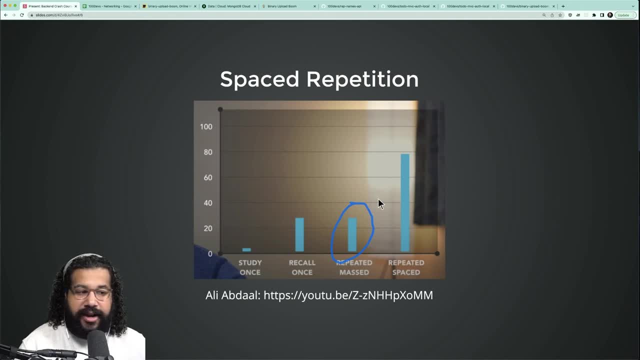 out your repetition. here's people that study just on saturday, and here are people that find time to get a little bit of studying in each day, right? so you're better off having an hour studying each day as opposed to five on a weekend, right? and if you can start, 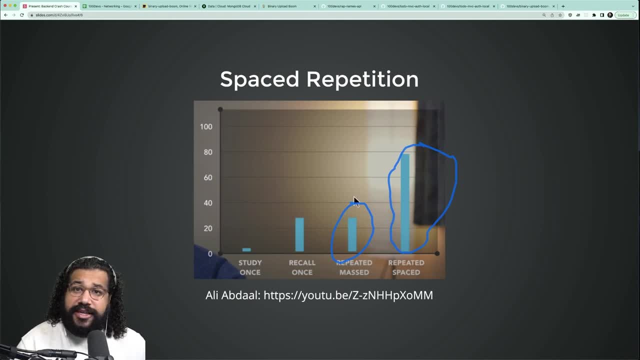 celebrating this space. repetition into your daily practice, just 30 minutes a day. you're going to see massive results when it comes to retaining information, especially with these like complex topics that we cover in software engineering. is there 100 devs? anki deck? there are tons of. 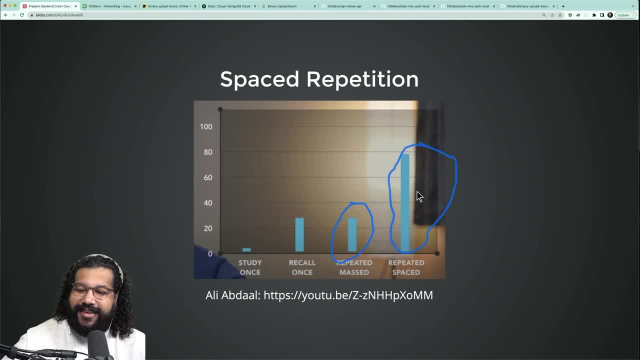 them floating around. don't use them. don't use them. why don't we use other people's anki decks? it's a really interesting question. the making of your deck is active recall. it is literally the primary thing that's going to help you learn right. so when you use other people's decks, you're depriving yourself of active recall. 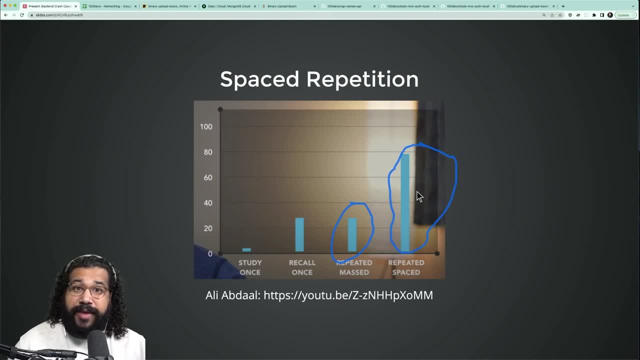 you're depriving yourself of a point of spaced repetition and we all remember things in different ways. right, and often tying the things you're learning to the process of learning them helps form the neural connections in our brain. so a lot of folks like to. a lot of folks like to write out their- i write out my- questions. there's some research that shows like: 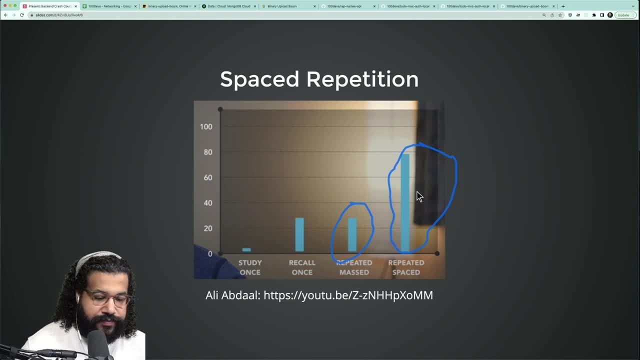 writing out stuff helps like remove your memory retention, and so i like to write out my questions to my anki and that process gives me active recall, gives me spaced repetition, gives me the benefits of having these questions and answers in my own words, right, and it ties it to the generation. 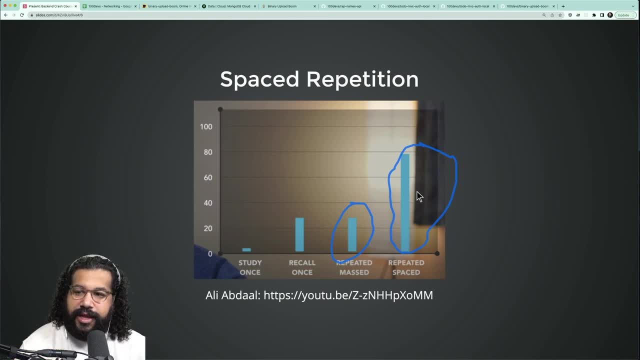 process, that my brain does something weird where i actually remember it, and so you could definitely find decks out. there's tons of them, right? but you're better off doing it yourself. you don't know how to read it, how to solve it, right? so there's a lot of things i want you to. 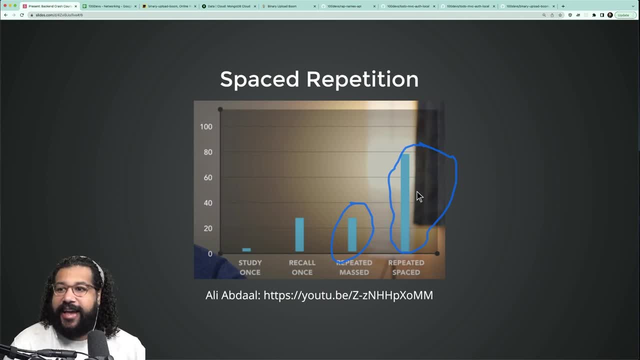 think about after you get started. and after you get started, i just want to remind everybody that you don't want to sit down and do an essay. don't worry, it's not an essay. you don't want to do an essay. you don't want to do it as a habit, and a habit is a habit, is an activity and practice. 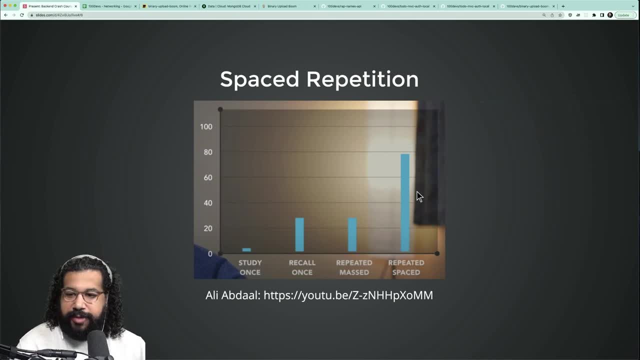 is an activity, so you're not supposed to be doing that. you're supposed to be doing that right. so, as i said, that being active recalling and training is not going to change anything at all. it's not going to change everything as you grow your ability to be moreми and get better. 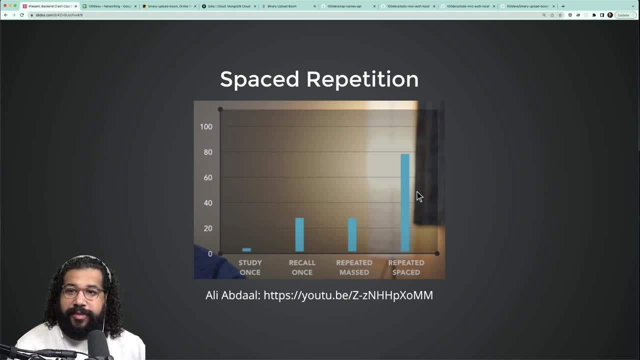 at those things you know. so it's not going to be a checked deck practice. it's going to improve. your best time is right, now, right, and so make sure that you're taking the time to do these things, because they are scientifically proven to work. they, they just work. having had thousands and 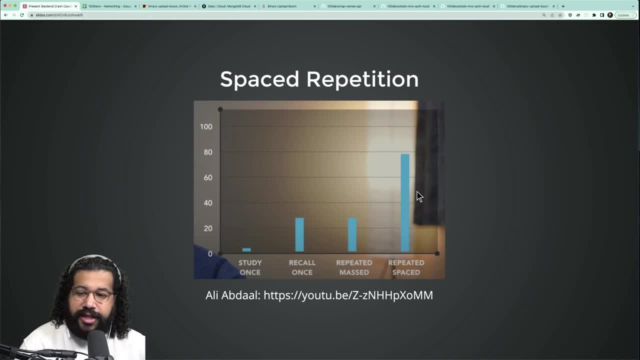 thousands of students that have taught how to code. there's two classes. there are folks that do the tools that help them to learn and there's folks that don't. and what's going to happen? what's going to happen is three months, like, let's say, you're brand new. it's the first time you heard. 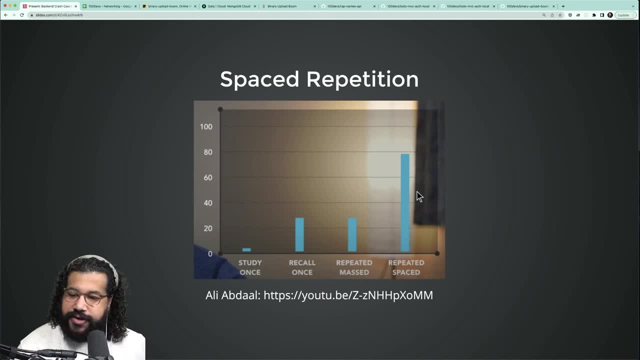 of 100 devs, right, first thing we've heard of 100 devs three months from now. you'd be like that was too hard i. i wasn't able to do it and you drop, right, you disappear. i guarantee you. the reason why you dropped and disappeared is because you didn't do active recall, you didn't do spaced. 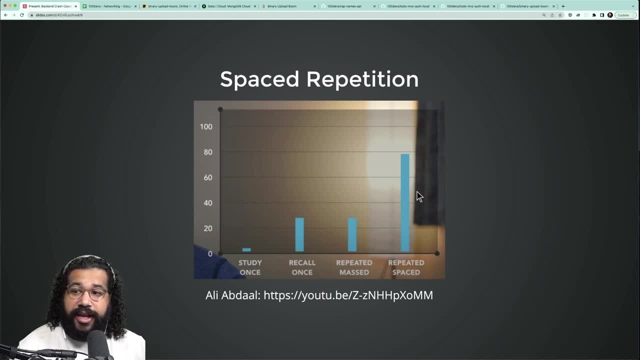 repetition: you didn't watch dr barbara oakley's course on learning how to learn and put that stuff into practice. barring life events, that's the reason 95 of the time you and you can even be here right now being like i'm barely hanging on to buy a thread. 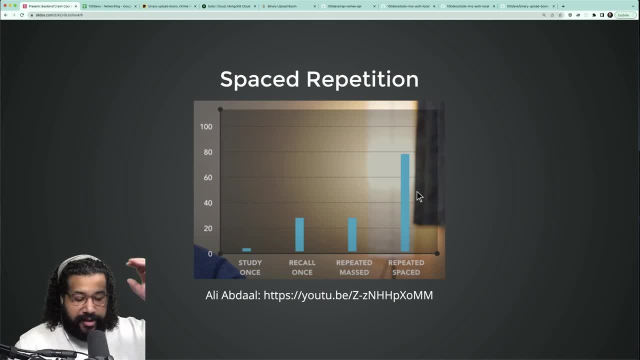 right, i'm barely hanging up by a thread, and the first thing when i'm so, i teach during the day, and the first when somebody comes to me says: leon, things aren't clicking, things aren't making sense. the first thing i tell them to do is show me your anki deck, and a lot of them go. 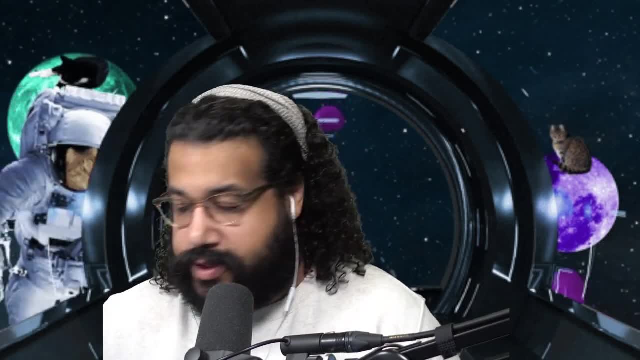 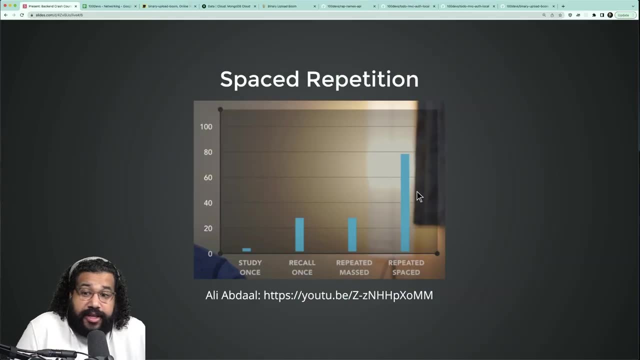 oops, right, and so you, you like there there's things that work and there's things that don't, and so what i don't want folks to have in the back like? learning the code is very, very hard. i honestly believe everyone can do it if they put good study. 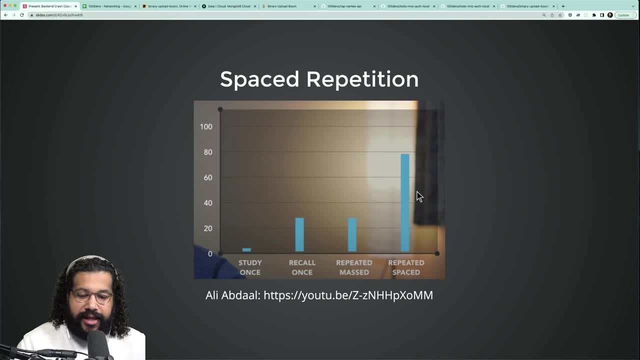 habits into practice, and i would say, barring, like i said, life events, right, some some, some, some learning challenges, that that that we, some folks, don't have the privilege of having, um, for, for most folks, it comes down to good study habits, right, and so, if you put these, 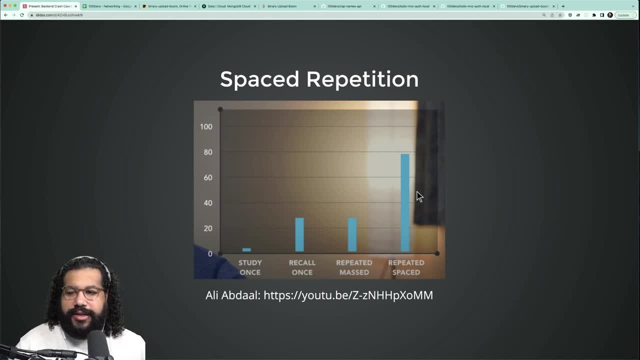 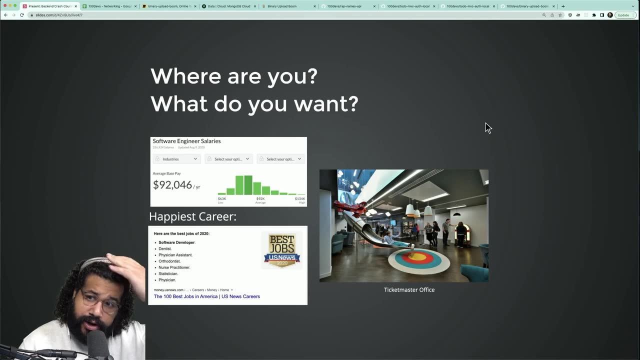 things in the place, i guarantee you're gonna have a better time. all right, so the other thing that you have to do is: because this is a lot of work, right, this is a lot of work and you gotta have a solid why, right, if you're gonna make it to the end, if you're gonna make it. 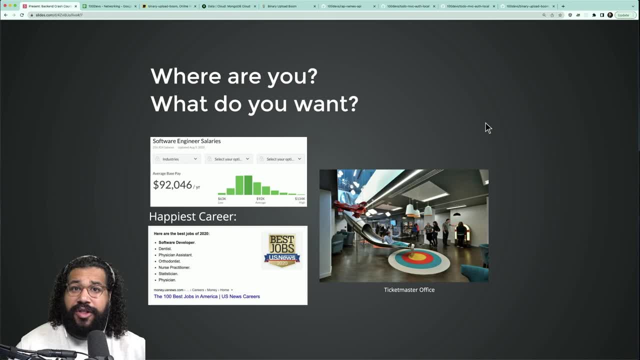 through the hunt. right, we're, if we're here, if you've been following along, you're here for a back-end review and you know you're gearing up for the hunt, to get the job. the hunt is a very difficult process. it tries you mentally, it tries you spiritually, it can shake you to the core. 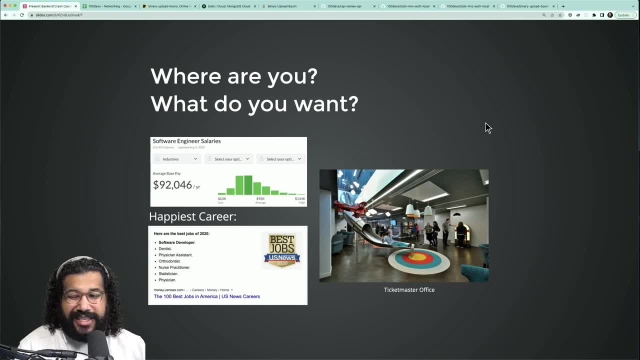 because it's rejection after rejection. when i tell you it's one out of 60, i really don't know. really do mean one out of 60.. we had war roach that said, on their 55th networked application they got the job. and so to put ourselves through that, you need to have a really clear why, right? 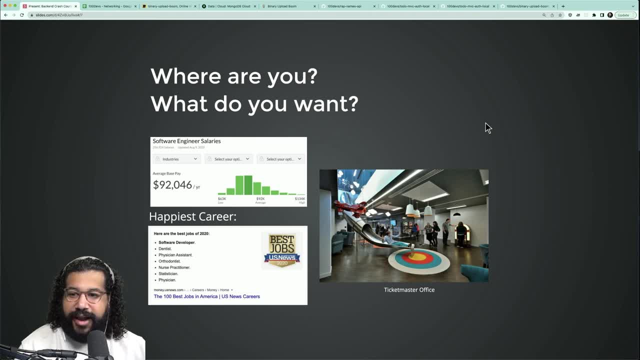 law says you have to have a prize to keep your eyes on. i 100 agree right. there's a lot of wonderful things about this career. it's high paid. it's consistently ranked one of the highest ranked companies in the world. it's consistently ranked one of the 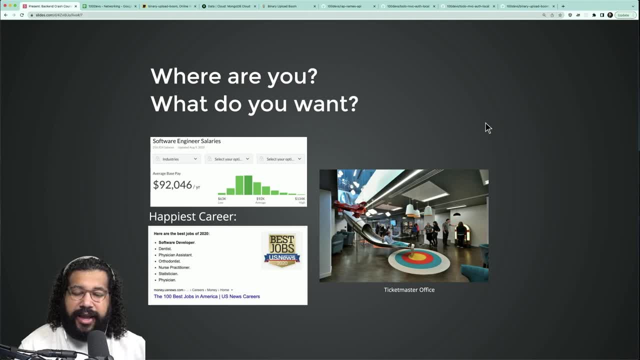 happiest careers. there's lots of flexibility to be had, remote, wonderful office spaces, sometimes with slides and arcades- like it's wild. i'm not a person that likes the hype fang like. you'll never hear me say, like go get a fang job. i think that's ridiculous. don't do that, because some youtuber 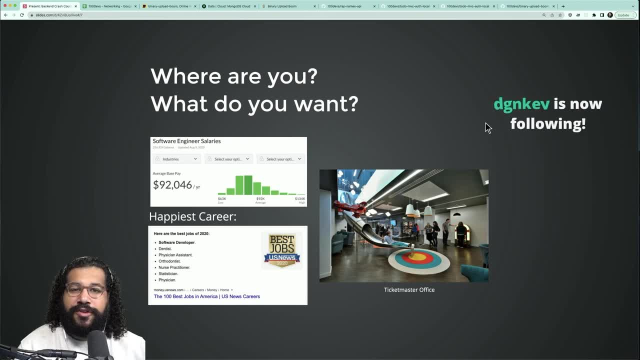 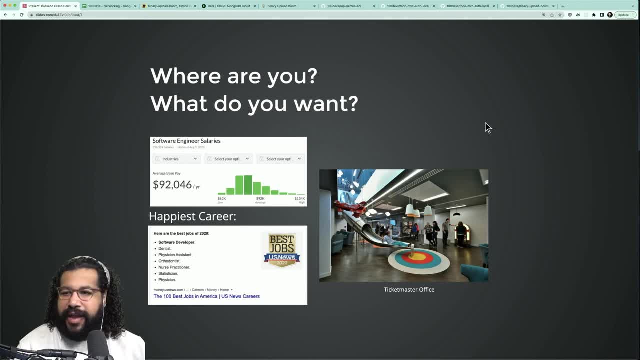 from home that you could spend time more with your kids and your family, right? like? there's so many, so many wonderful things about this career. it's fun, like building shit is fun, right, you could be working on building projects that you love, and so there's something here for everyone, um, and you. 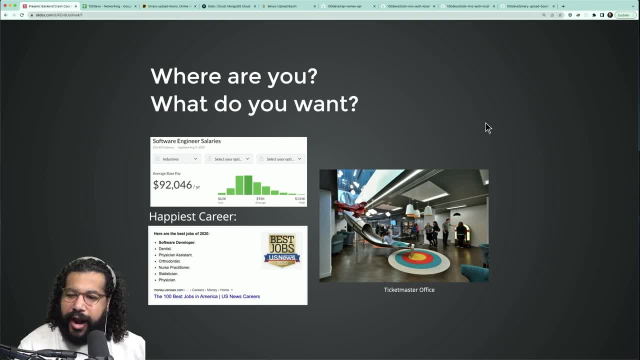 really have to focus on your why. why are you putting yourself through this? learning to code is hard. why are you putting yourself through the wiggles of false hope? that is the hunt. what is your why? like, you need to think about it, and you need to think about it, and you need to. 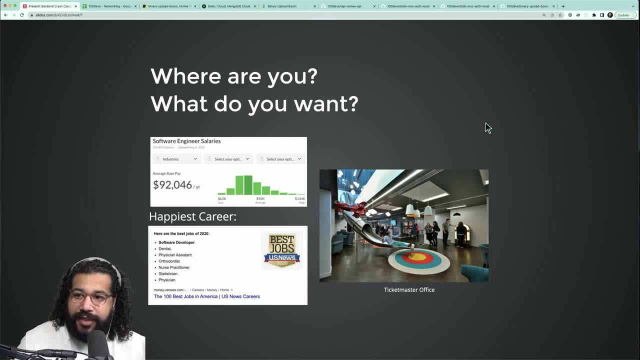 think about that right now, like when we take our first break. while you're getting your water, you're hydrating, you're getting up if you're able to, and walking around. i want you to think about what your why is right, like: keep that in the back of your mind. why are you giving me six hours on a? 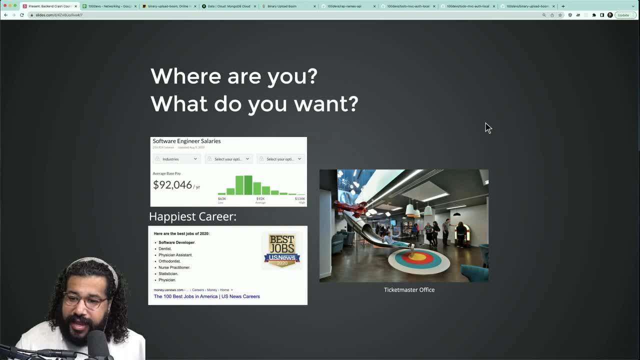 sunday right. why? and if you can focus that. why i guarantee learning to code. it's easier. because when you're lost in the sauce, it's not you're lost in the sauce, it's. i'm gonna get there. because why? because i have to, because i want this thing for my life. 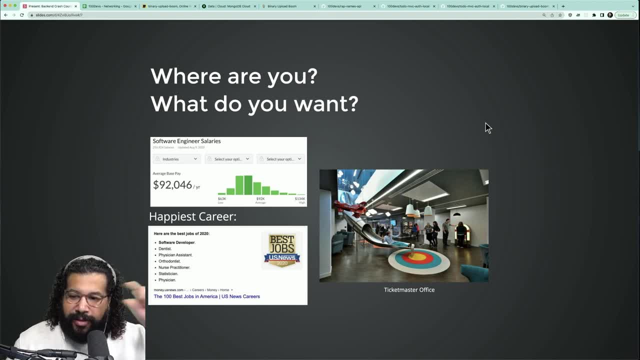 right i. i want this for my family. i want this for my future. i want this for i don't care, i want the porsche i. i don't care what it is like. whatever that that motivator is for you, you gotta have it, you gotta. i have a lot of folks that just put like a sticky note. 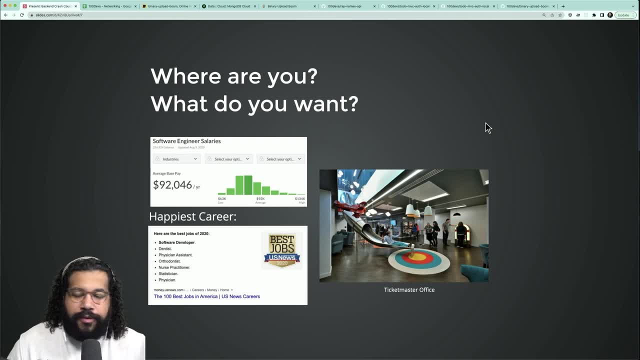 on their monitor. right, right, what is your why? why are you doing this? right, it could be that you just love to build cool shit, like. whatever that why is? it has to be front and center, or else this process will tear you apart, and so a lot of folks when it starts to get a little stressful because they're not centering. 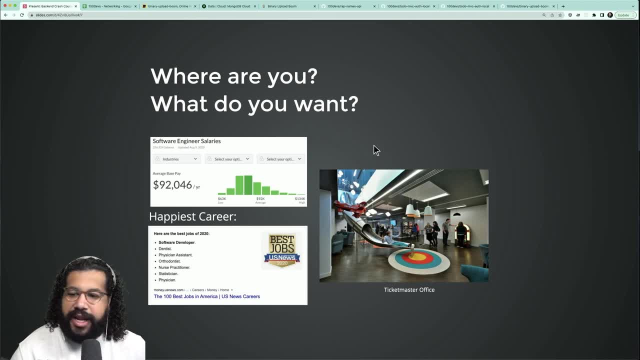 on the why right, like: who cares if it takes me an extra week to learn something? right? who cares if it? if, if i don't understand something the first time i cover it, i'm going to be like go to my wolf, right? who cares if if, if my first three rejections come through during the hunt? 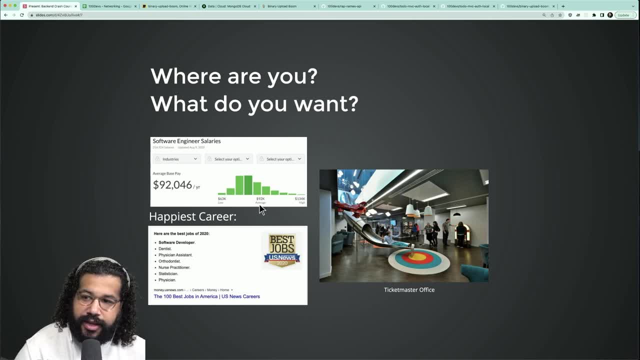 i'm sticking to my why, right, i'm sticking to my why and you gotta have it. don't, don't continue with this program without a why and it could be the. it doesn't have to be that deep, doesn't have to be that deep. i love programming because when i looked at my bank account, money was there. 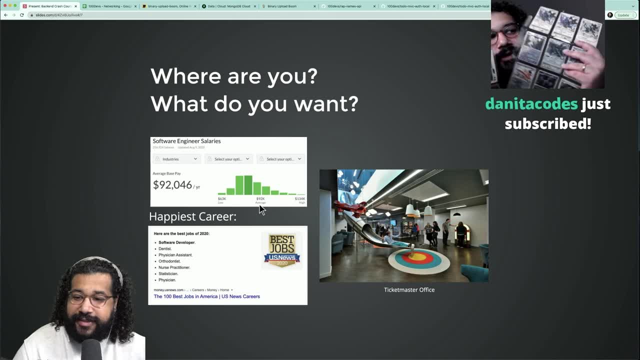 that's why i love programming. that's it. that's where i started. i started with that why i want food. i want food. that's literally why i started coding, because i wanted food. right like, figure out what your why is and there's a chance to grow into it, to turning into something that 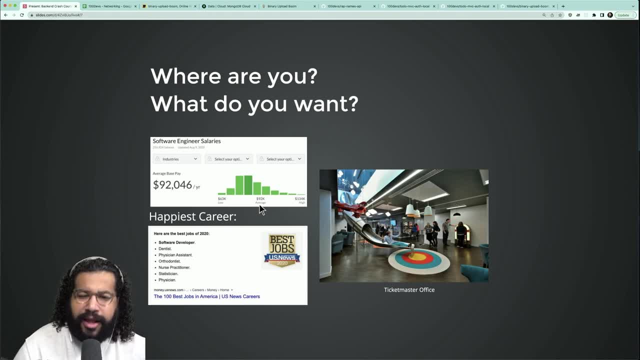 you love, right, i love learning about code, i love writing code, i love building cool shit every single day. but it didn't start that way, right, it didn't start that way. don't ever let somebody tell you that you're not good at coding. you're not good at coding. you're not good at. 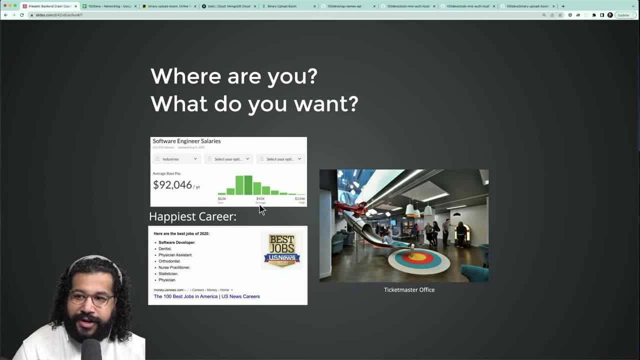 that you have to. you have to be in love with writing code to be a good software engineer. nah, the best software engineers i know, clocking at nine, leave at five. they don't touch code on the weekends and they're beasts. right, right, but figure out what your why is center that you're. 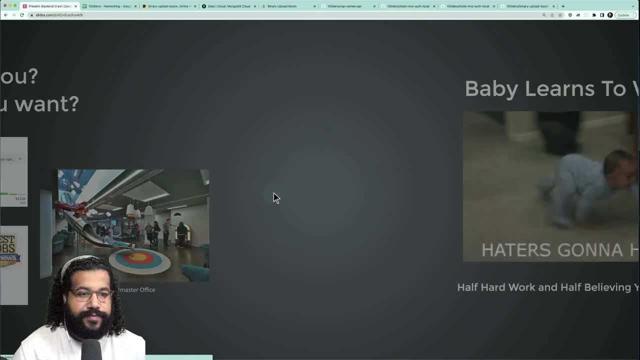 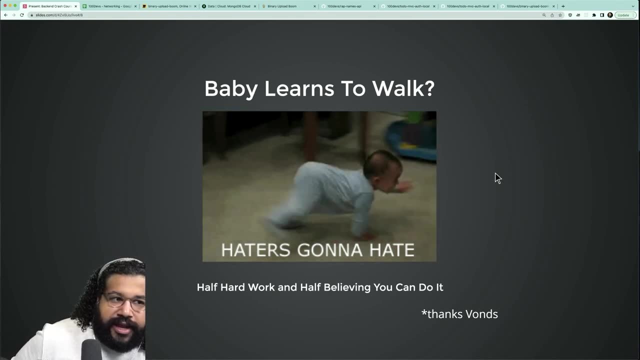 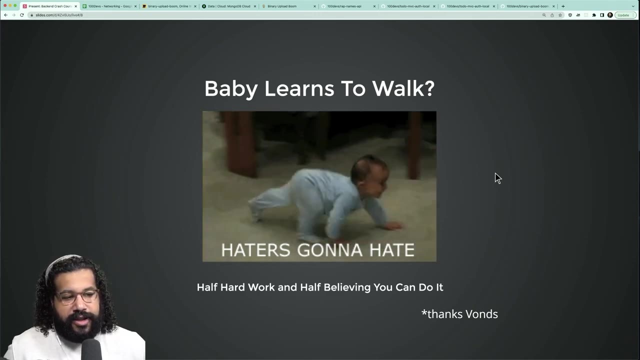 gonna need it for the rest of the program. now, one of my experts and residents at resilient coders that i work with every day had this great knowledge. i had this wonderful analogy that i think is super important and it they relate it learning to code like babies learning to walk. 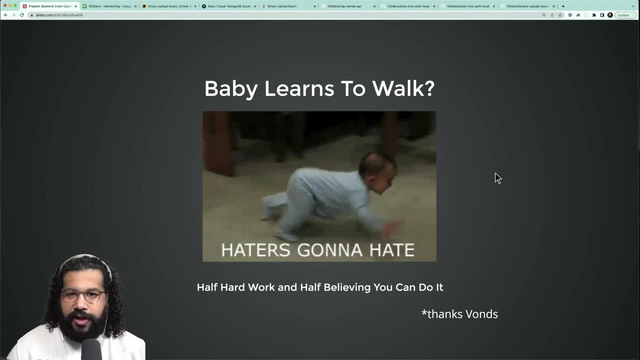 babies learning to walk is half like hard work- like them getting up, falling down constantly, not being able to do it, and half believing that you can actually learn to walk. so, babies, look around And they don't start crying and sitting in a corner, going: I'll never be able to walk. 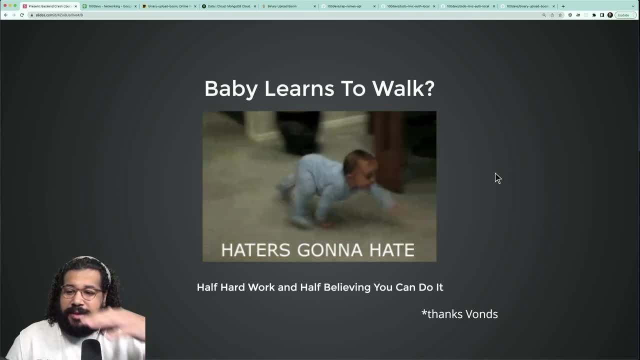 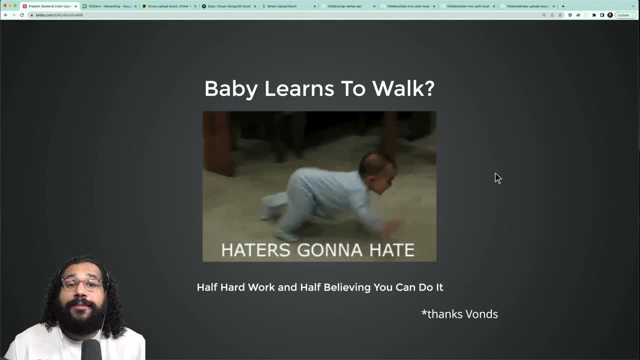 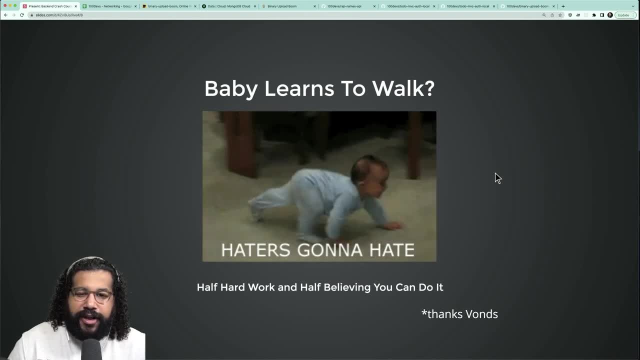 having a better grasp of node. Don't ever look at those people and go: damn, I'm never going to be able to do that. That makes absolutely no sense. You have to believe, Right. You have to believe that you're going to get there too. 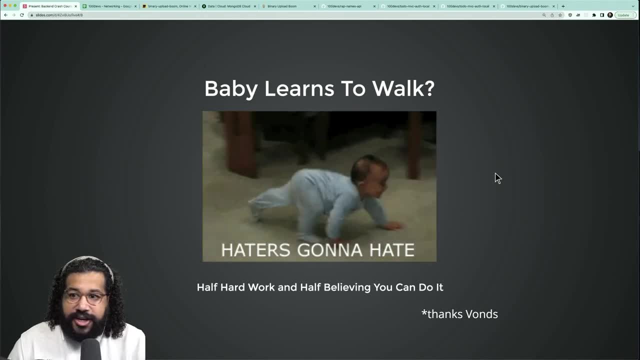 And, if anything, seeing those people walking is should be the biggest highlight of your day, Cause you're like, if they can do it, I can fucking do it too. Right, I think so many people see, see folks walking, see folks getting jobs. 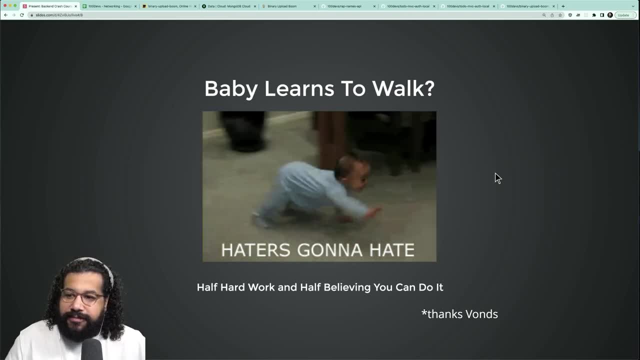 They see folks picking up concepts And for some, some reason in their brain, in their body, their soul, they go. I can't do that, Cap. You all have the ability. You all have the ability. It just takes a lot of hard. 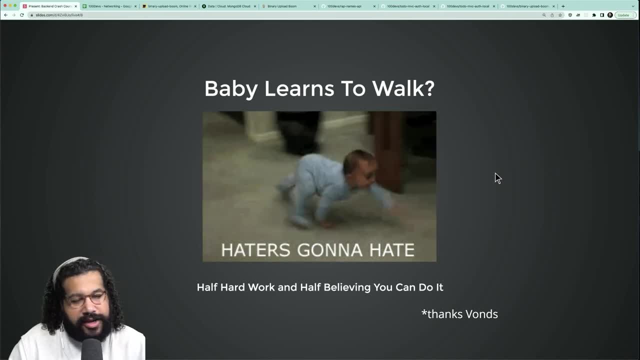 Work and babies don't sit in the corner crying. Sometimes you need a good cry, but babies don't sit in the corner crying. What was me? I'll never be able to do it. They see everybody else walking and they get up, they fall down. they get up, they fall down, they get, they fall down. 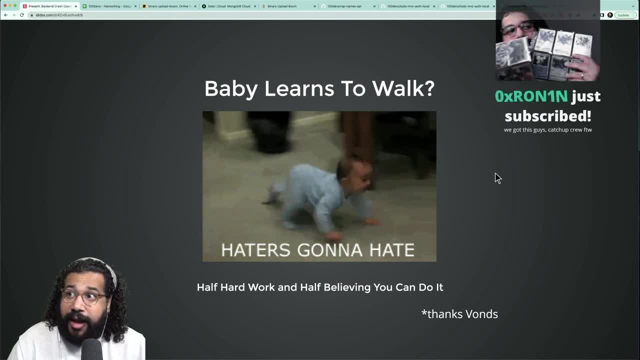 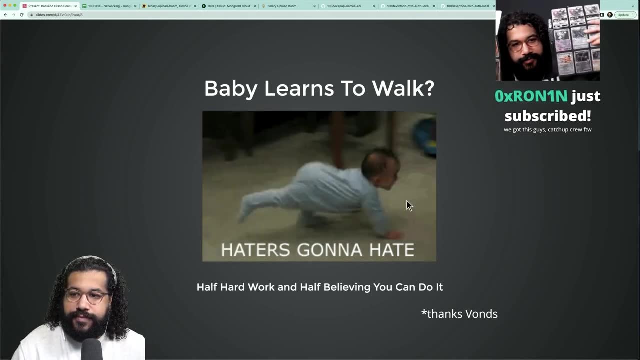 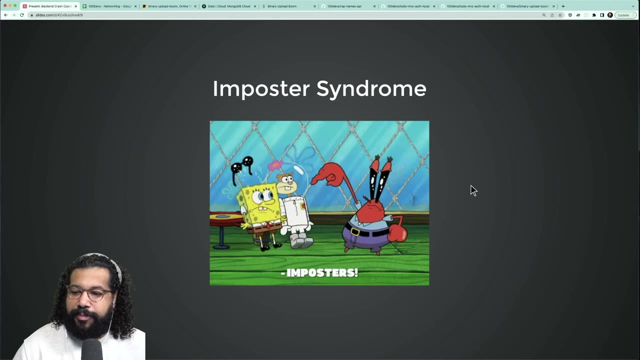 So you need to get up and you need to fall down a couple of hundred more times and you'll get there. Yeah, Yeah, Yeah, Yeah, Yeah, Yeah, Yeah. get there too. this is also the point of program where imposter syndrome becomes probably your. 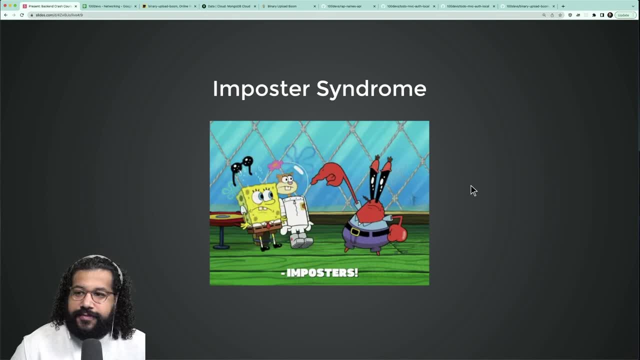 chief, your chief concern. I think this is the point of program where imposter syndrome comes in the full effect and this is honestly what will hold the most people back from achieving their why all right, and getting getting the shit done. like I said, you see other folks starting to get jobs and for some people that 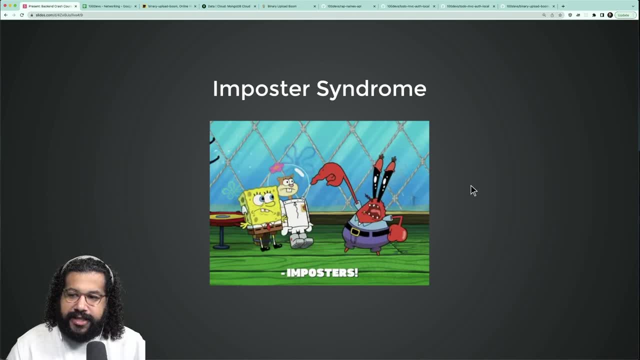 trigger something in their brain that makes them feel like they can't do it too, and you need to squash that. that's that. you just need to get rid of that right now. it's just absolutely not true, other people. success takes nothing away from you, nothing from you, and you have no idea. 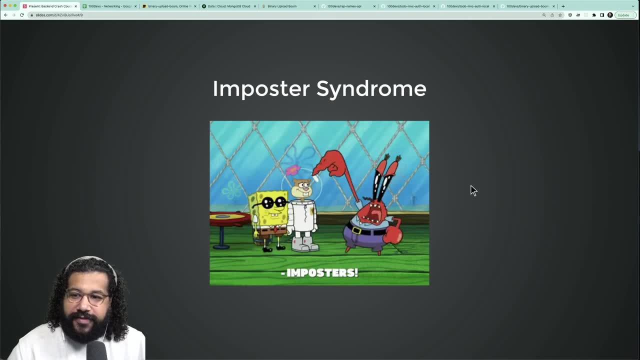 you how long they waited to get on that front of the car. You have no idea what experiences they have. You have no idea how their life is set up right now to do all this. You can't look around at other people walking and think that you won't get there too. 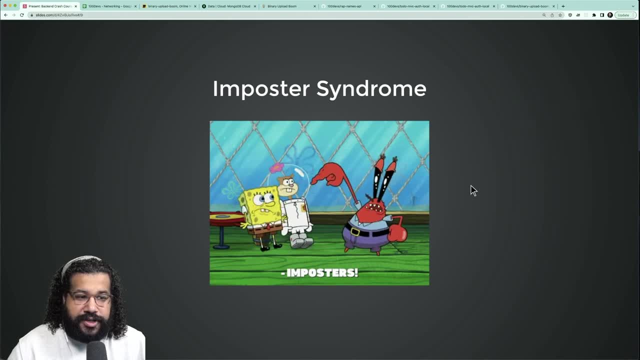 Babies, don't do that. You don't do that Now. the other part of imposter syndrome is: we're getting close to the hunt, Right, Right, We're getting close to the hunt, which means that you're going to now have to start. 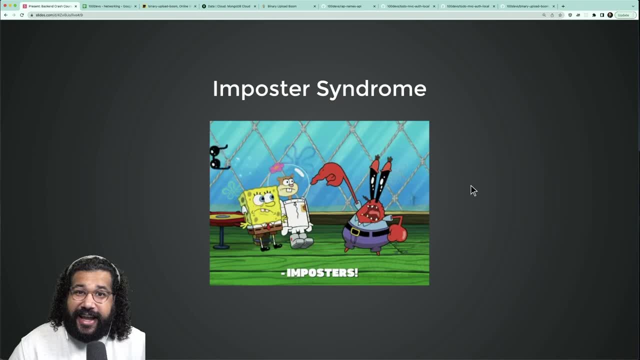 showing others that you can do the things that you can do, And that triggers a whole other level of fear within ourselves. But that's why it's a numbers game. Right, It's 100% why it's a numbers game. You're going to have 10 interviews that go horribly wrong. 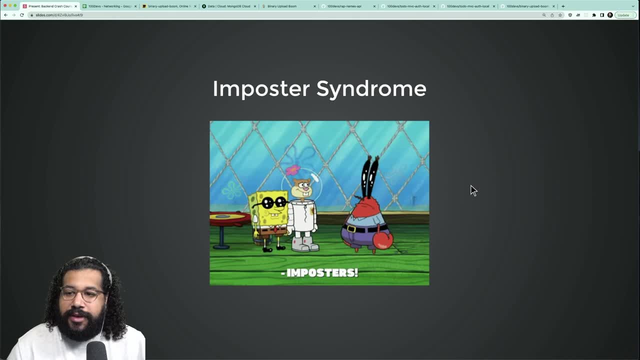 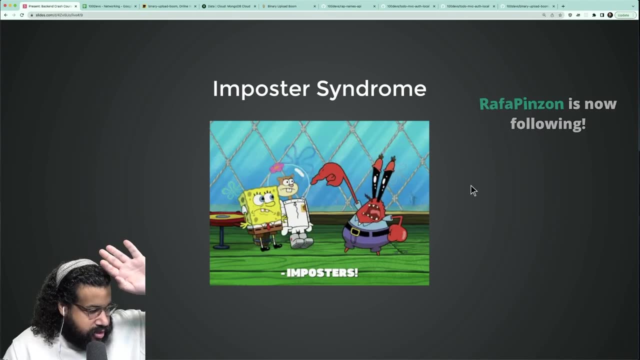 Like you vomit on your keyboard, You slip Right And as you're slipping on your vomit you're like I don't know I'm trying to think of- like the worst thing that could possibly happen: You hit the nuclear launch codes. 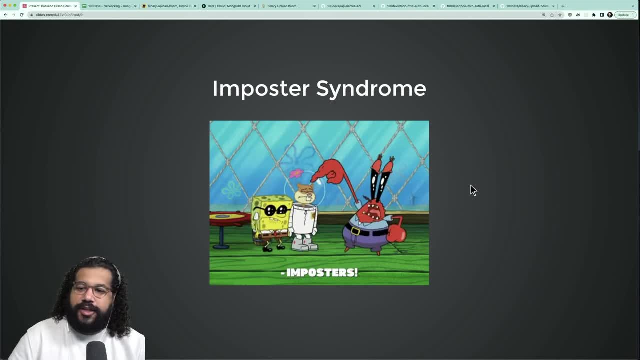 Right, I don't know. Right, You do something horrible, Like it's just going to go, like the worst thing you could ever think of, Right, And so what you have to realize and you poop yourself on the way down. 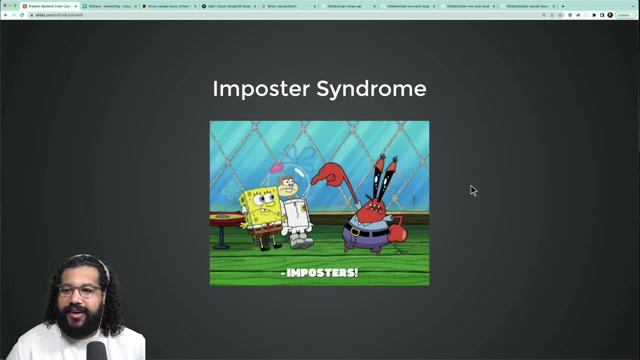 Exactly, Nerd On the way down. You just have to realize that Every single one of us has 10 of those in us. Every single one of us, Every single one of us has 10 of those in us, Right? 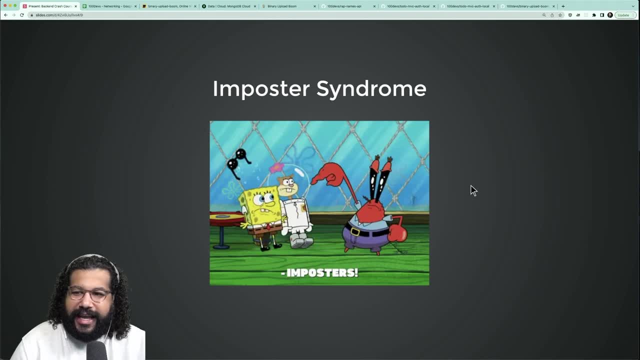 Right. And so you can't think less of yourself when I'm telling you You already have 10 of those in you, Right? And then you got like 40 mid-interviews, Right, You got 40 that are going to go, eh. 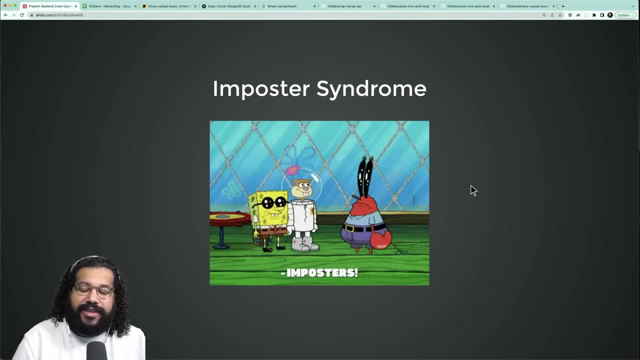 Eh, I was there. It kind of went okay. And then you'll have 10 where the stars align. You're going to feel like all the planets are in direct alignment with you. You're going to feel like Like I don't know. 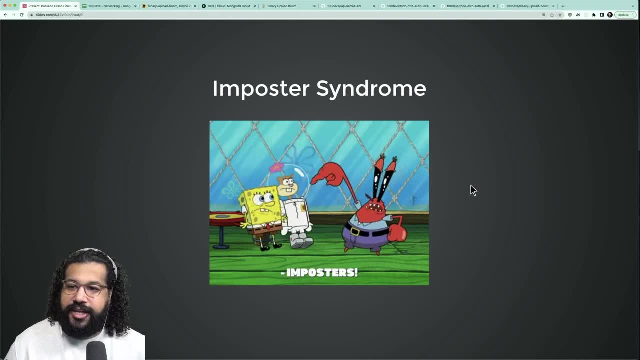 That somebody was whispering all the answers magically into your ear. It just happens, It's a numbers game, Right? And so you can't let the nerves get to you, You can't let the imposter syndrome creep up, Because it's just the fear of the unknown. 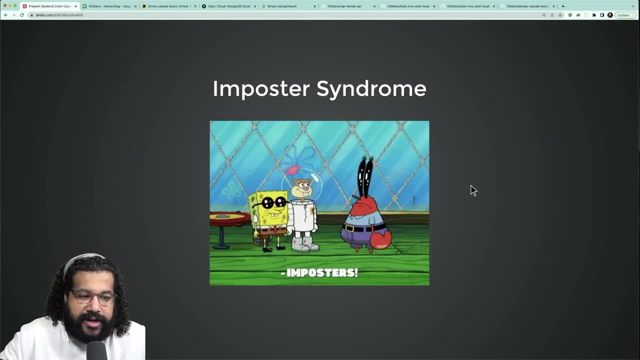 It's just the fear of what if somebody is going to ask you Like it just doesn't matter. Right At the end of the day, All these companies that you're going to join are going to do things in their own way. 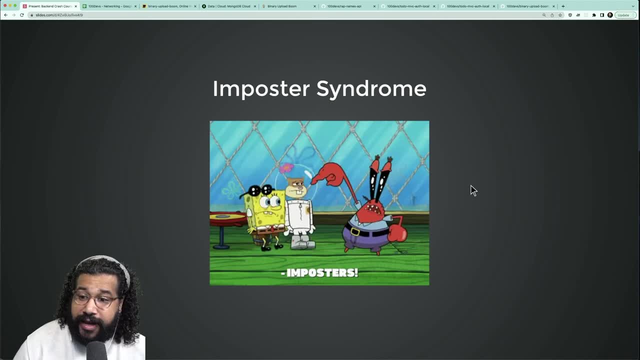 And they're going to expect you to take three to six months to ramp up. Most companies expect you to take three months to figure out what the heck is going on, Right, And so you're going to learn just enough to get your foot in the door. 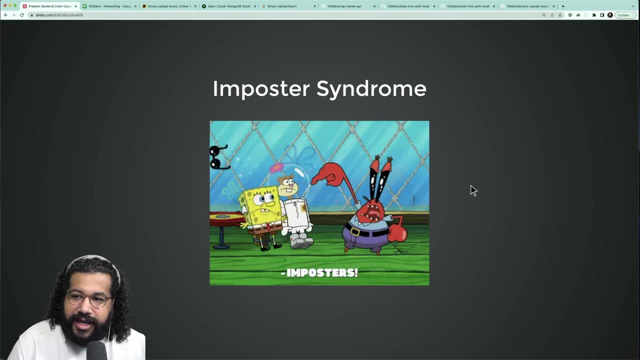 And then you're going to work your ass off once you're there And worst case scenario, Worst case scenario- you get paid for three months to learn how to code. Let's go turn up, Right. And so the imposter syndrome. 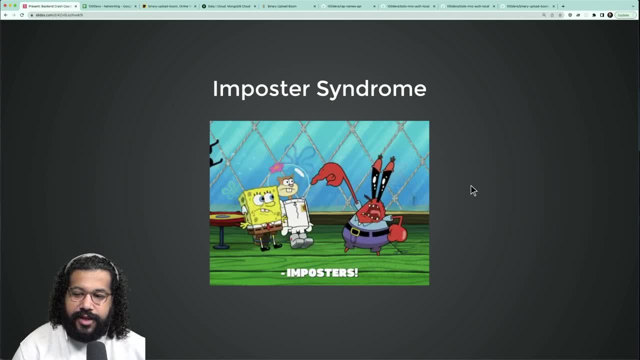 This is when it hits. It's not warranted. You've been putting in the work, You've been here, You've been showing up, You've been building your projects. You've been doing the things that you need to be doing to get these jobs. 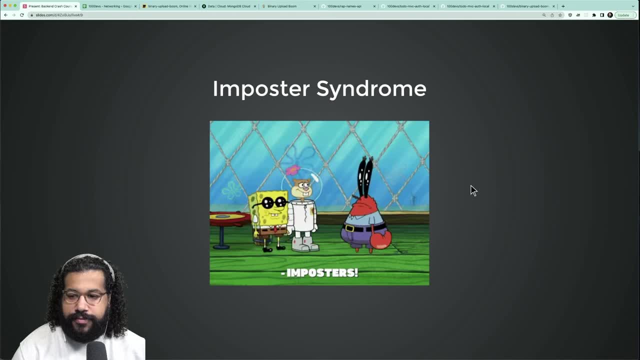 You're a great software engineer, Full stop. Now it's time to find the right fit for you. It's time to find the right interview process for you. Every company does it differently. There's going to be something that clicks for you and the things that you know. 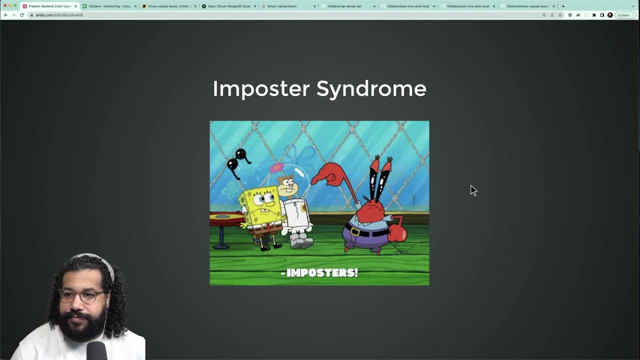 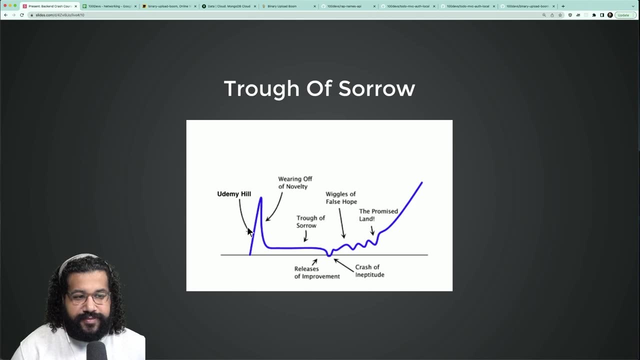 And you'll be an asset to that team. So I'll be most looking forward to it And everything seems to be going well. since you put it in, I've definitely been wanting to get into design. You do this when it's on. 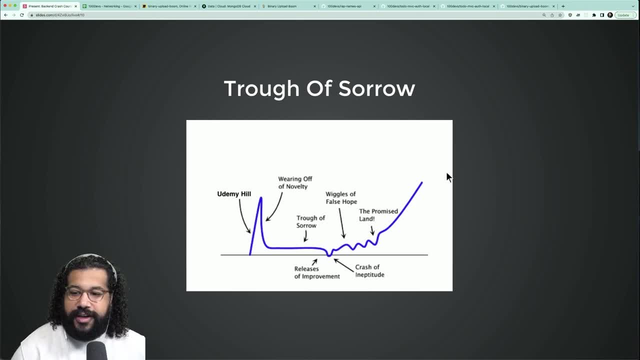 You just I'll do it next time, because that's what I've been meaning to do every year. Okay, Tried to find my life. I'm forward to that. Finally, I like the之 e filter. I use it a lot. 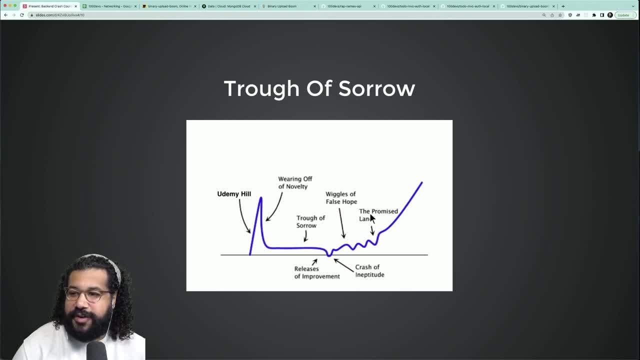 You know I might move out after I'm done. You're not going to recognize it, You'll do it right. You already witnessed it. You always feel the Peace Trap and all that And feel like you're a brand ambassador for this's show. 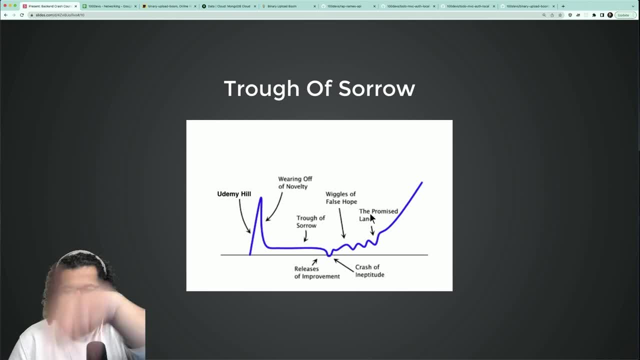 So I've been doing this every single day. I never stopped. I'm kind of done: right now, right, and then a week later they're like fuck, that was true, and uh. and so i i think the uh, the trough of sorrow is very real, right. i mean, most folks aren't willing to sign themselves up. 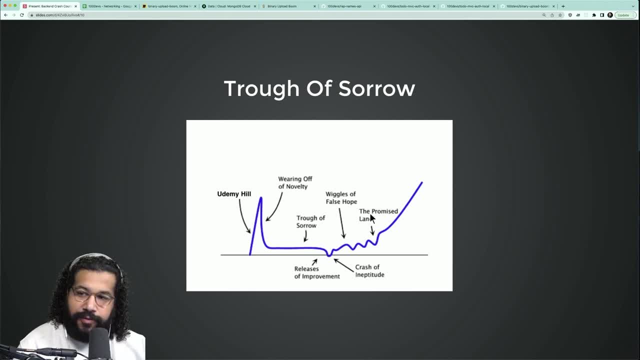 to go through six months of sorrow, right, they're just not willing to do that, right, because, like that it's just. it's just, it's six plus months of sorrow, like most people in the world aren't willing to do that, and, uh, i think our, our, our, our community showed that right, like we started off. 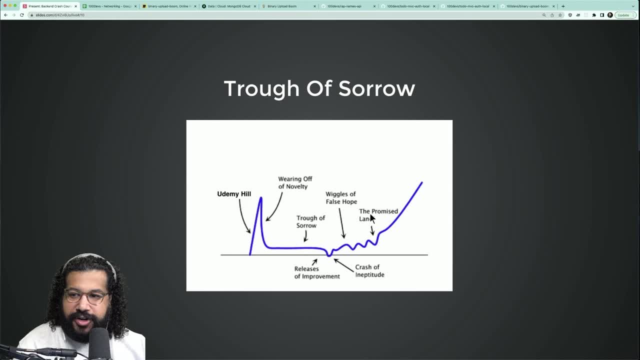 with uh first class, which is always a scrub because people trying to figure out what it's going to be. but our first class was 5400. right, like after the, after the, the intro, like this is what you're signing up for? 5400. and now, now we're we're at like one to two thousand, right. 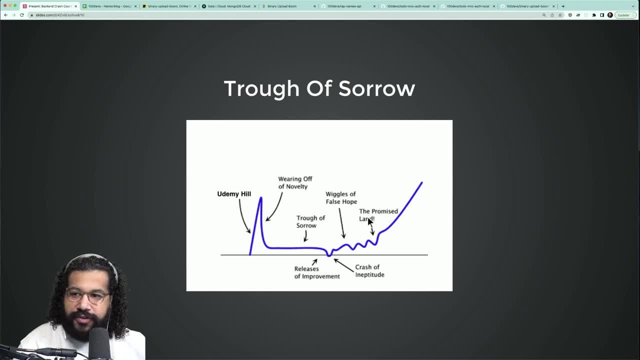 like we've kept a strong number of folks. but this trough of sorrow is real right, is real right. you get stuck right. you get stuck in this trough of sorrow right and most folks don't want to work through it. right, right, right, right, the more you do it. 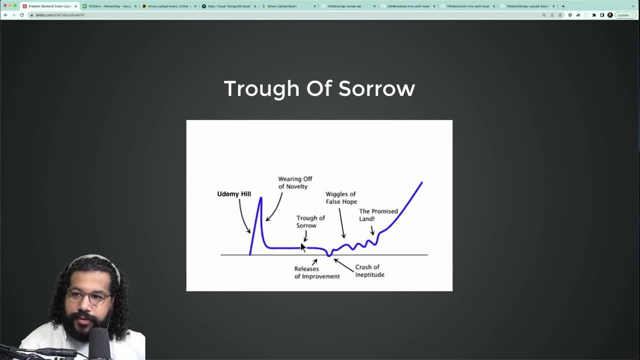 right. the more you do it right, the the more you trudge through it, the worse it gets right. the worse it gets right like the this, this trough of sorrow, you, you, still. you're still like in the fun part. you just went down the roller coaster, you're like foot, and then you get to. 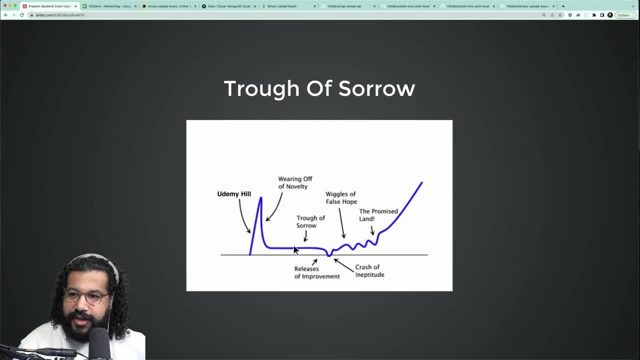 the bottom right. this is the real trough of sorrow that that, three months in, things still aren't clicking right. things still aren't clicking. you're, you're, you're feeling, uh, you're, you're, you're feeling the all the insecurities, you're feeling all the things that are that are coming up like. 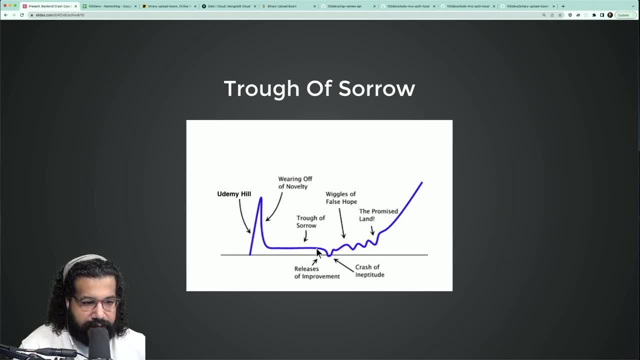 that's the real trough. and then you've pushed it. you've pushed it to here and now we're building full stack web applications and you're seeing folks get jobs. and then you tank. everyone does it. this is the process you tank. there's something about being close to the end that messes with us. it's the worst part of 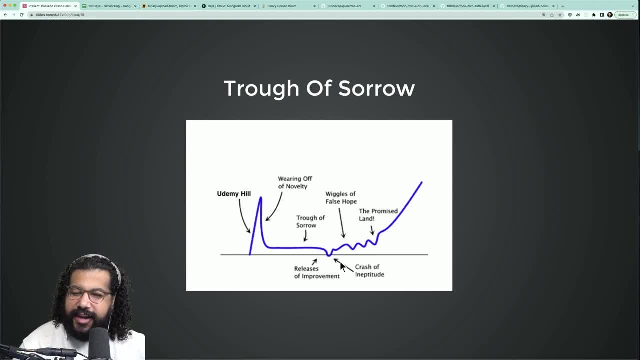 the process. when you're so close, you can see it. you're seeing other folks around you- all the imposter syndrome comes through, right. all the imposter syndrome comes through all of the the struggles of realizing shit. i got real deadlines. holy crap. like this stuff i really need to start. 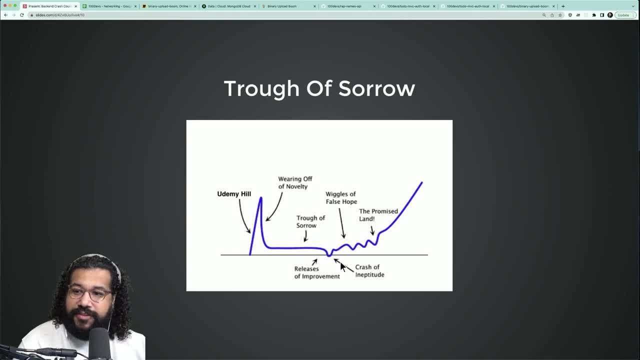 putting into action. i'm gonna have to start talking to people in these interviews like all that stuff. i'm gonna have to start talking to people in these interviews like all that stuff comes together and that's why this little dip right here exists. the worst part is where most 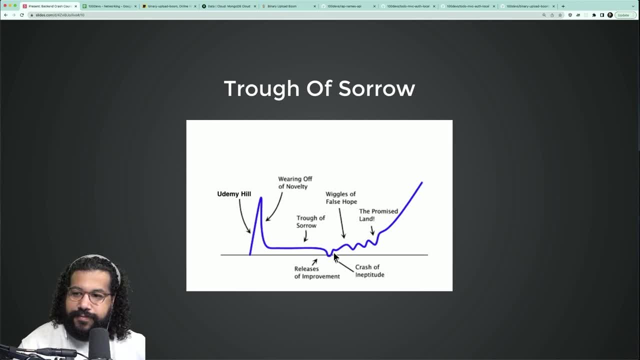 folks take themselves out the game. and then you start to. you start to build your hundred dollars project. you start to realize that, wait, when i build up that checklist, i'm starting to get recruiters reaching out. right, i'm starting to like, maybe understand some things. i have to. 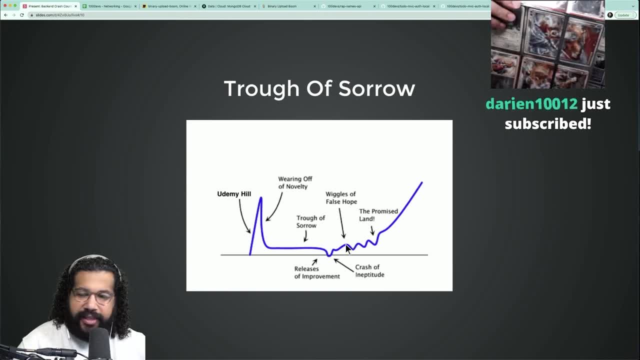 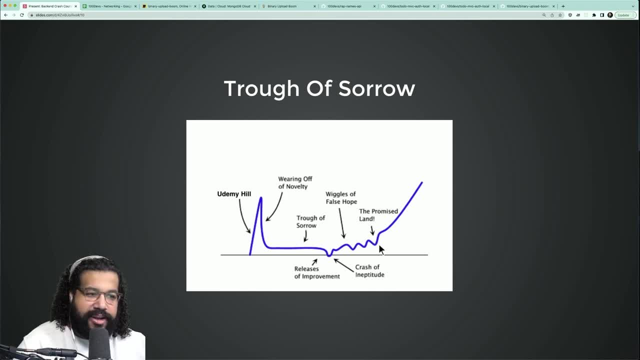 interview and it kind of goes well, and then boom down again, interview down, interview down, interview down, up and down, up and down, up and down, sideways, left right, boom, boom, boom, boom, boom. and then eventually the stars align, that one interview goes really well and you make it to the promised land. 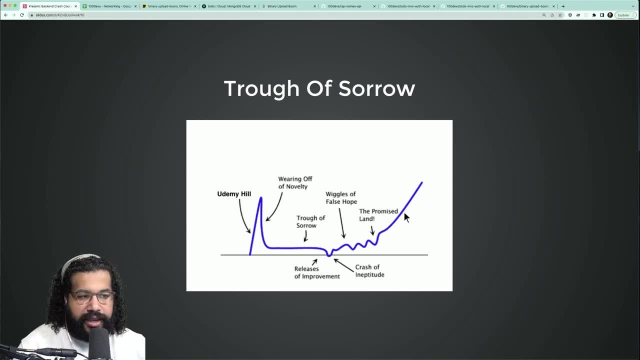 and then you're out of the trough of sorrow. you still fight and you fight over the next rest of your career to keep learning and keep growing. and you're out of the trough of sorrow. you still fight and you're out of the trough of sorrow. you still fight and you're out of the trough of sorrow, you still. 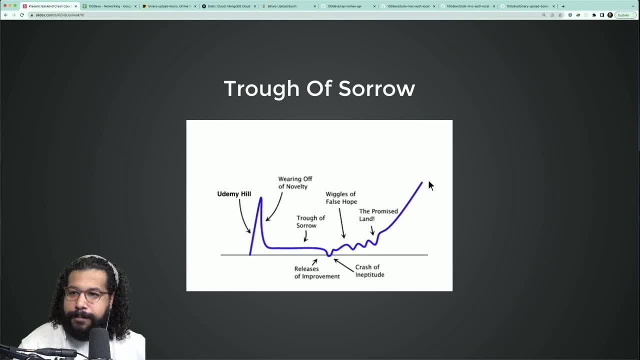 growing right, right, right. so don't realize that most of us are right here and realize this is the most difficult part, where all of our knowledge is coming together to build full stack applications. all of our doubts are coming to the surface, because now it's time to start applying stuff. 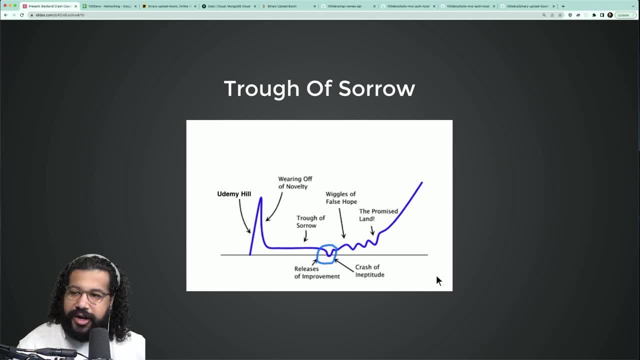 all the the judgment and worry that comes with the interview- and this is the hardest- is part, but we'll get there as a community, right? we'll get there as a community. as you need help, come to discord. leon noelcom slash discord, right? if you're watching this on youtube, 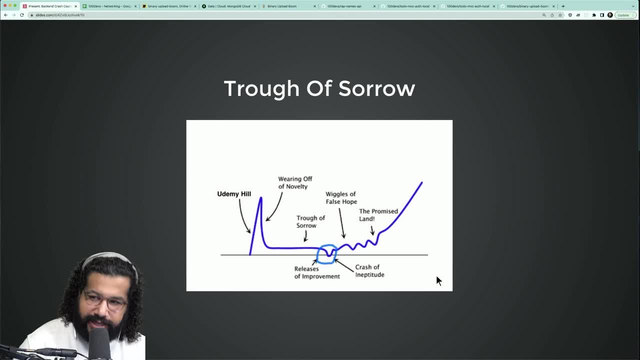 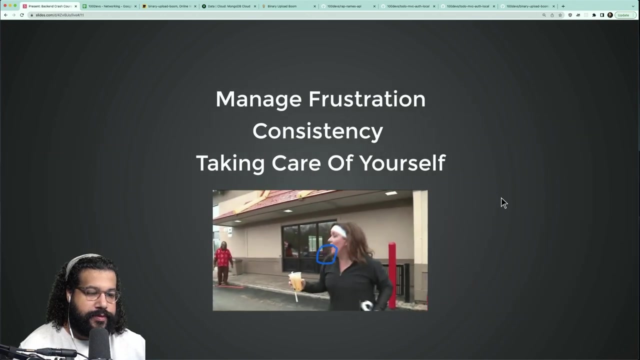 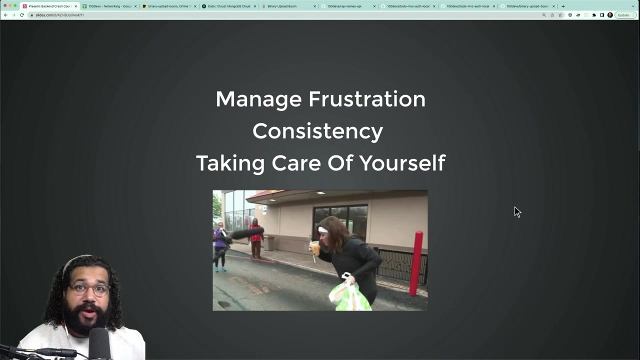 discord. if you're brand new here, exclamation point discord. you can do this. you can absolutely make it through the crash of ineptitude and into the wiggles of false hope and into the promised land. cool now before we jump into the rest, before we get into basic javascript. 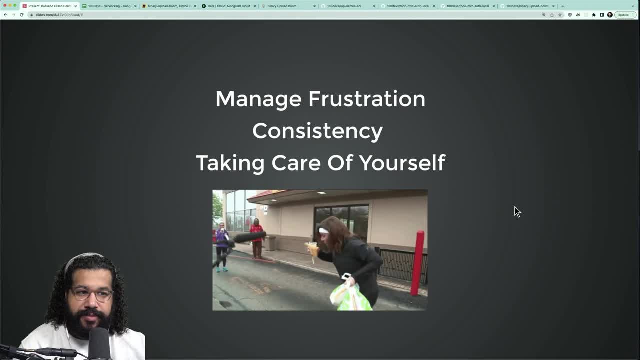 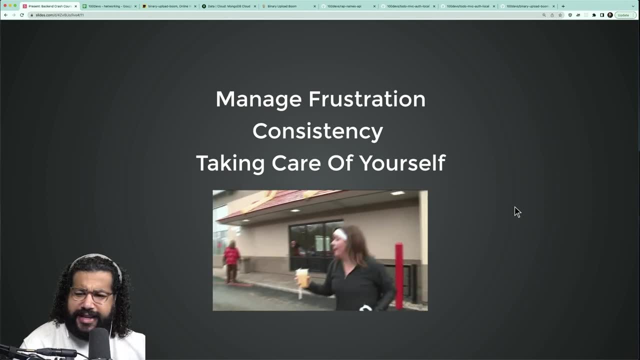 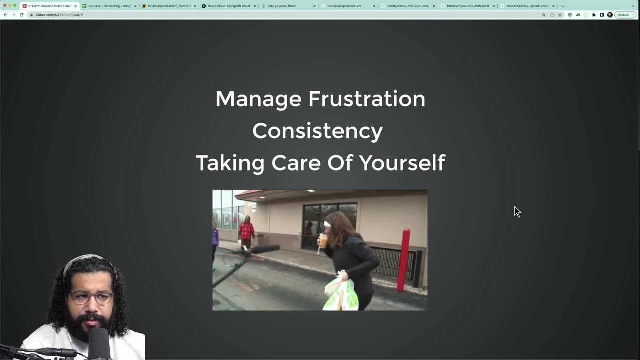 right before we in the basic javascript: three things. this is it. i, after thousands of thousands of students, i can say tens of thousands of students now, with 100 devs, um, um. managing your frustration, being consistent and taking care of yourself are the only three things that get you to the end, the only. 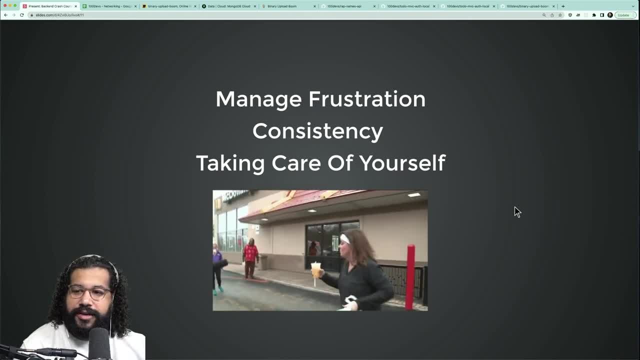 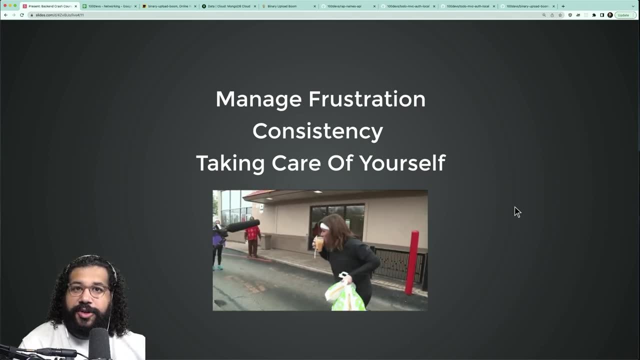 only three things that literally help you get the job in the end. I've talked about the studies in the past, about the magic frustration. Basically, they look at you, look at adult learners. The reason why adult learners don't actually learn how to code is because 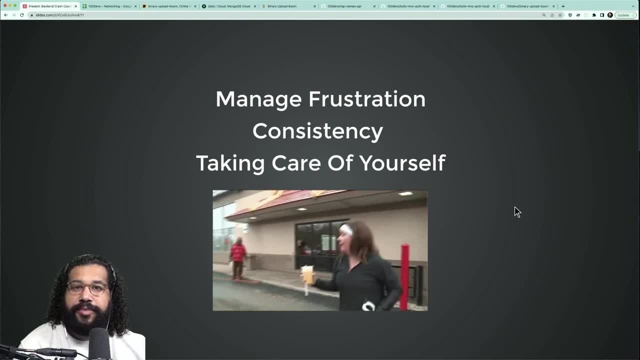 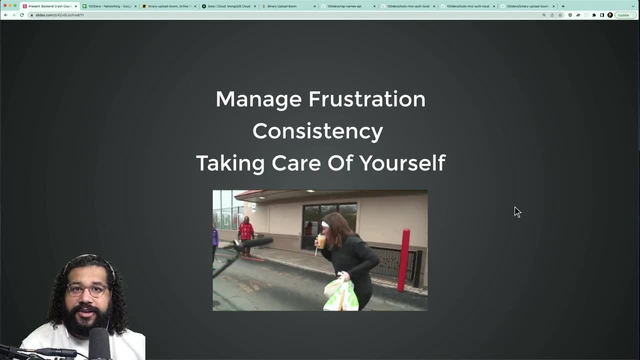 they are in control of their life. They can decide to put Netflix on instead of studying, And so when things get tough, when they get frustrated, instead of doubling down and trying to get help and working through it, they turn on Netflix Right. 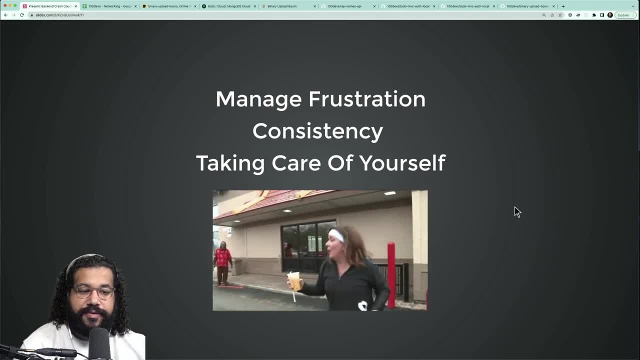 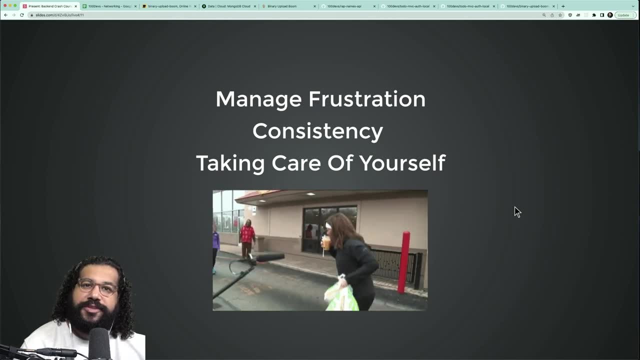 And so the more you can manage your frustration, the easier it is to learn. and managing your frustration just starts with realizing that you're frustrated and coming up with systems to not be. That's it. It's coming up with systems to not be frustrated. 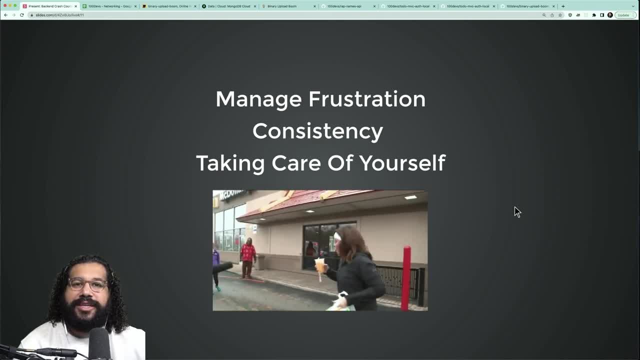 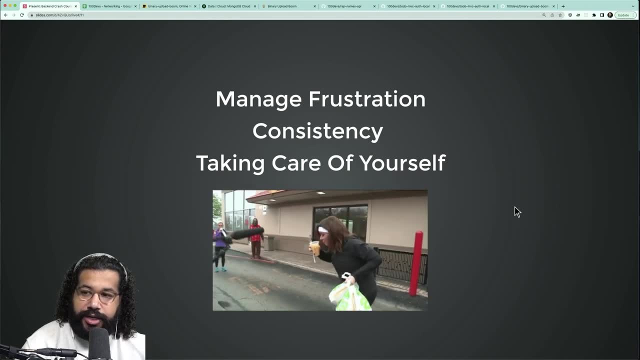 So for some folks that is all right. When I'm frustrated because I'm stuck on code, what do I do to get unstuck on code? Do you? do you post on discord? Do you jump in a voice channel? Do you ping folks on discord? 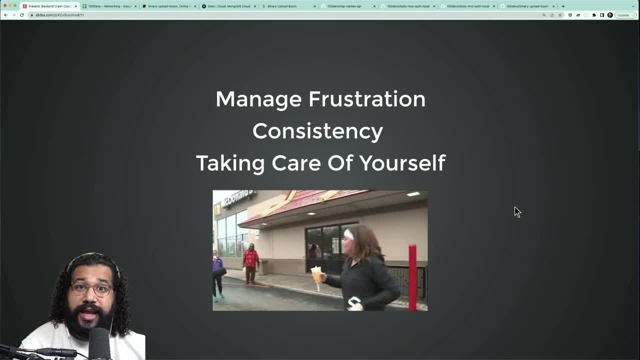 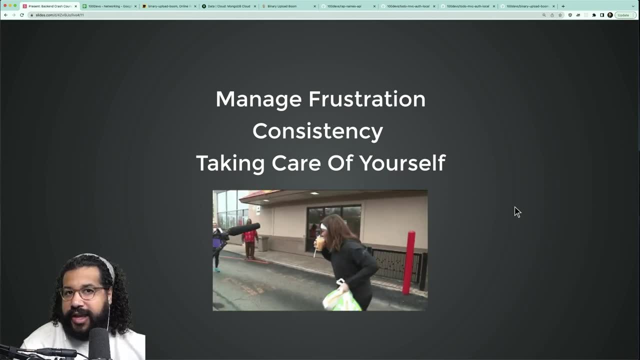 Do you go to the stream- team members streams- and ask they're like: what do you do to get unstuck? So your frustration subsides and most folks don't have a game plan for when that happens. But if you put a game plan in place for that, 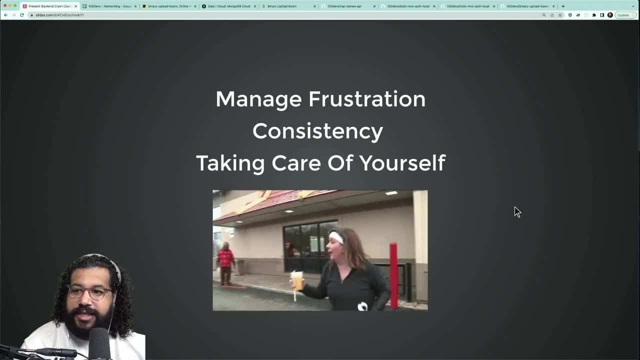 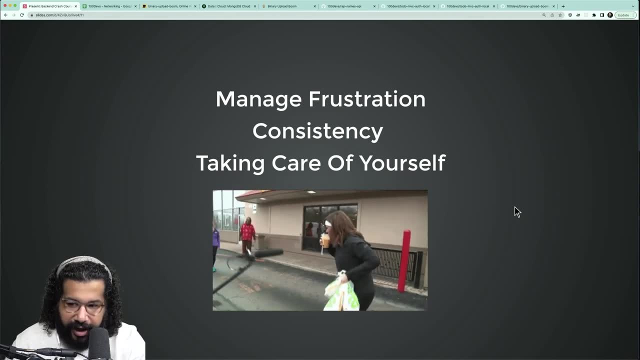 because a little easier. the next thing is being consistent. Consistency works because we saw that spaced repetition works- Literally scientific fact how adults learn. spaced repetition is the key to not forgetting stuff. It's the key to learning stuff is active. recall is the key to getting that. 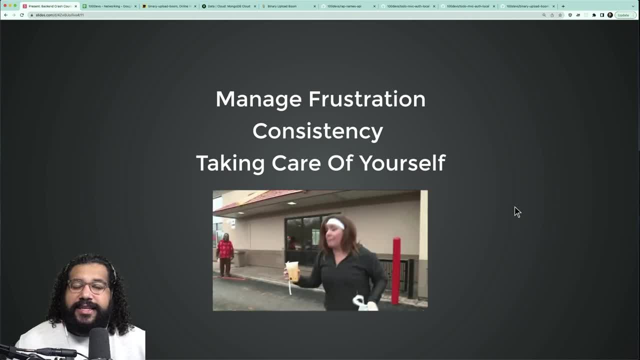 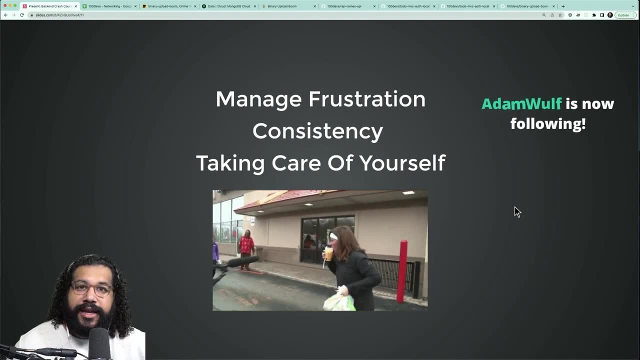 material in with a quarter of the effort. and consistency means that you can't just chunk one day of the week and hope that you remember something a week later. doesn't work, It's daily practice. It's squeaking out 30 minutes a day. 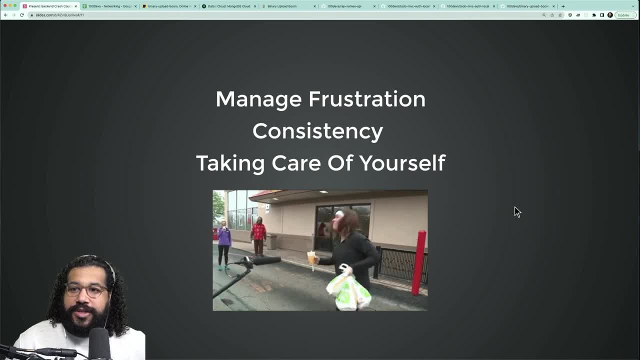 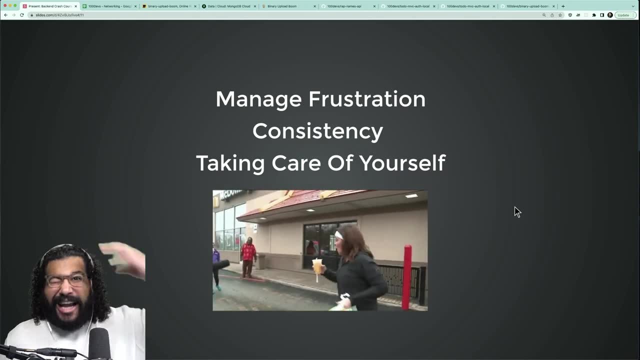 So you can get that spaced repetition in right, So that you can, so that you can reap the benefits of the things we know actually help you to learn as an adult. And then the last and most important thing is you're signing up for months. 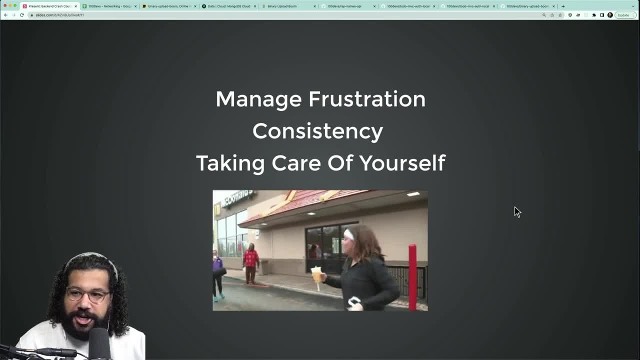 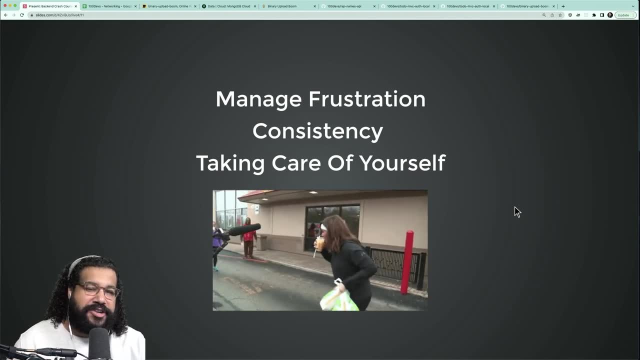 and months of mental anguish, making your fingers on the keyboard, do things you haven't done in a long time, sitting for long hours, staring at screens for long hours, constantly getting rejected When you go into the hunt. it's a lot. 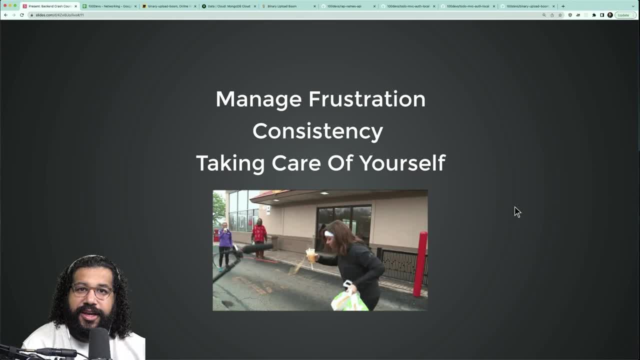 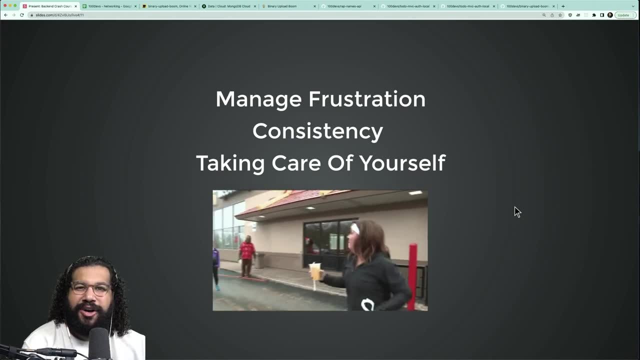 You have to find ways to take care of yourself. You have to introduce breaks. You should be doing Pomodoro, right? I know a lot of folks like to, to, to just go for three, four hour stretches. I'm telling you. 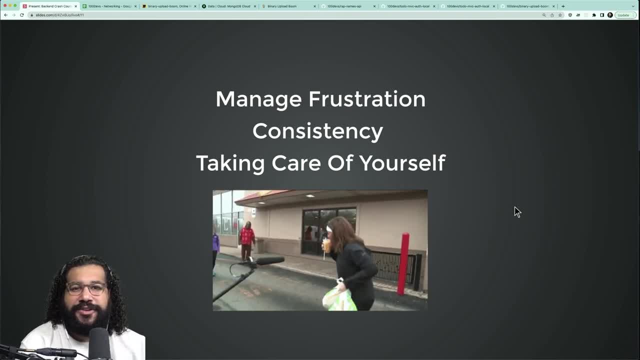 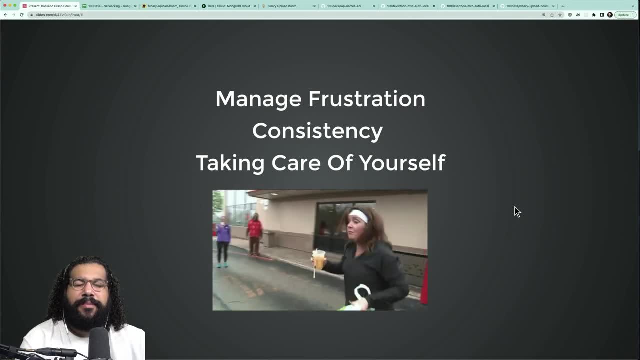 if you do that for months, most of my students are not successful. doing that- Taking good breaks, taking care of yourself, hydrating, walking away, letting your brain diffusively think- pays off to significant dividends. We're not in flow states yet. 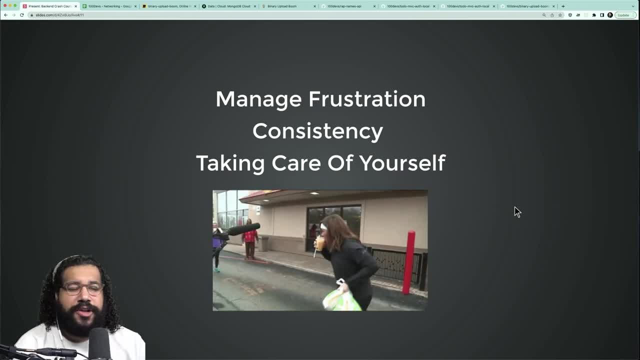 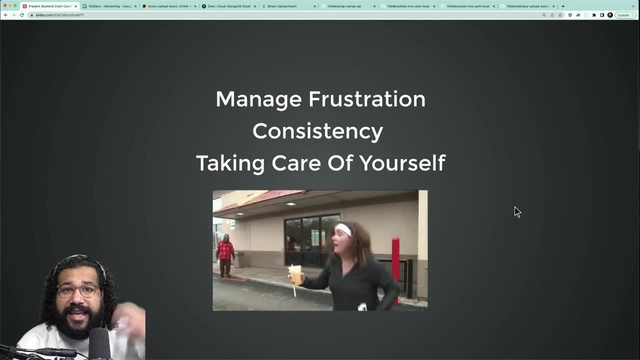 right, We're in. We're in learning mode. When you're on the job, maybe you'll achieve flow and you can code out four hours straight. That's fine. right now You're learning And we know the research behind memory consolidation. 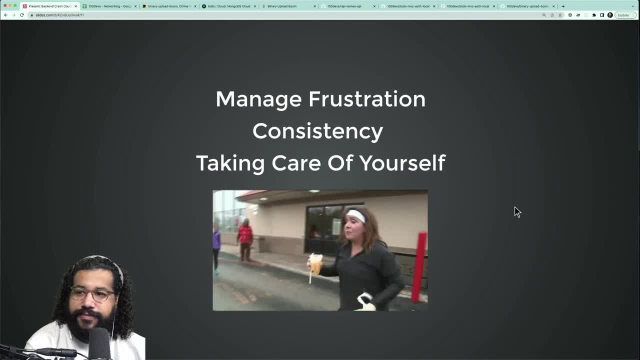 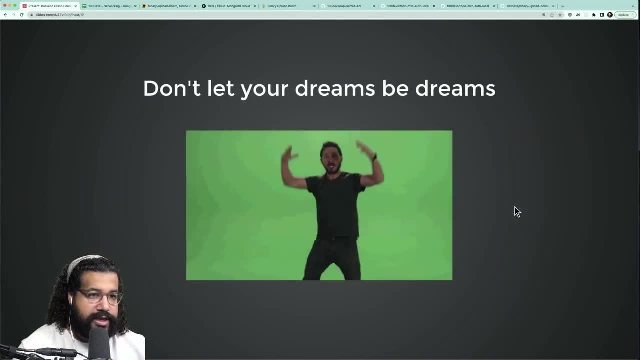 and it doesn't happen. when you do it for that long, You need to take breaks, Cool, So, last but not least, uh, don't let your dreams be dreams. Do it, Just do it. So just do it, Just do it. 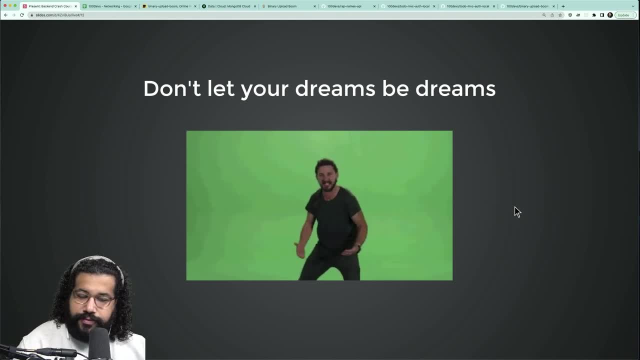 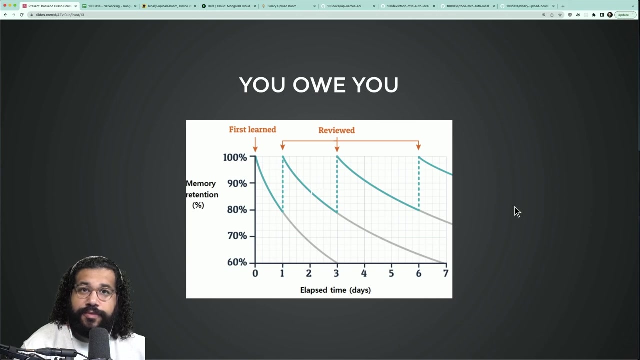 Make your dreams come true. Just do it. All right. Center your why manage your frustration? be consistent. take care of yourself. You do that. You make it to the promise Lynn. you owe you. you owe you. I can't make you do anything. 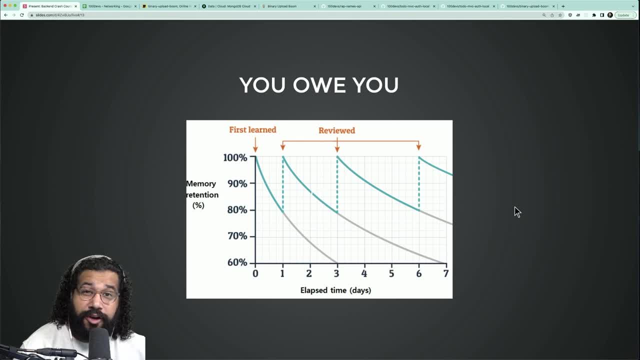 but you deserve a high paid career. You deserve a happy career, You deserve a flexible career. You deserve the things that come your way When you put in this amount of hard work, when you put in this amount of supporting those around you that are part of 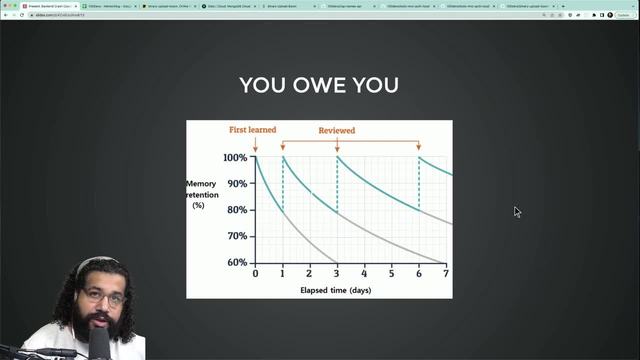 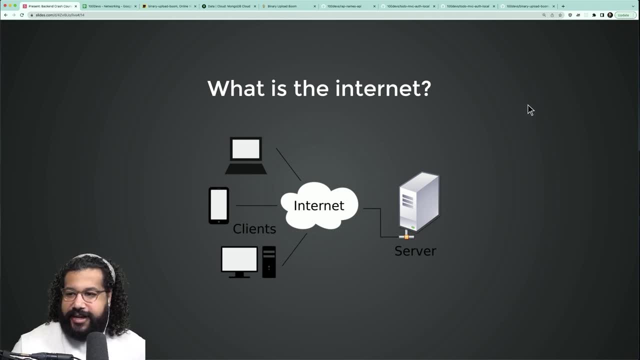 this community. you owe you. What is the internet? Bring it all the way back. What's the internet chat? What's the internet? It's a wire connecting two different things. It's a wire connecting two different things. It's a wire connecting two different things. 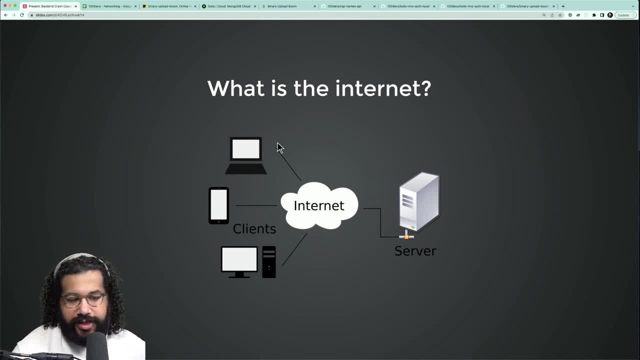 It's a wire connecting two different kinds of devices. We have our clients- So think of our desktops, our laptops, our mobile phones- and they were make requests to servers. Their servers are just computers out there on these internet wires that can hear those requests and respond. 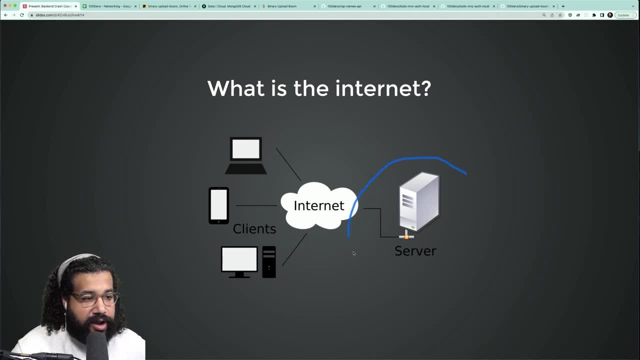 Eventually, we are going to be writing code that exists on these servers that can listen to those requests requests, generate the responses and then respond right, And so the beauty here is that we can build out applications that look good on our client-side devices, and that would be our. 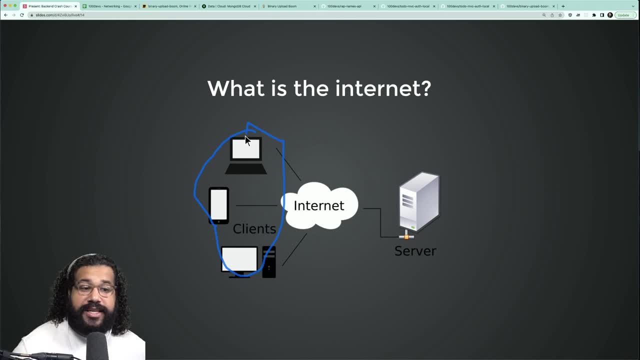 front-end web development, So building out the HTML, the CSS and JavaScript to make our stuff look good and run good on these client-side devices. And as backend developers, we can write the code on our servers that listens for requests and knows what to do when it hears those requests. 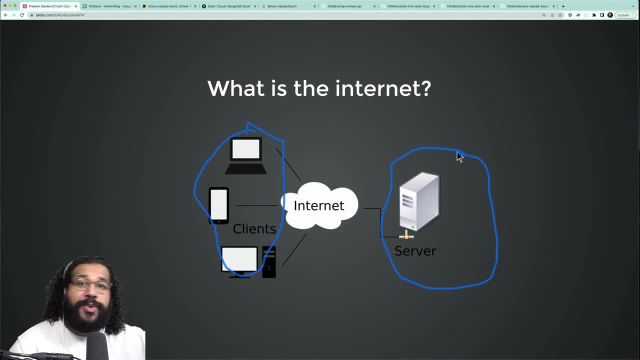 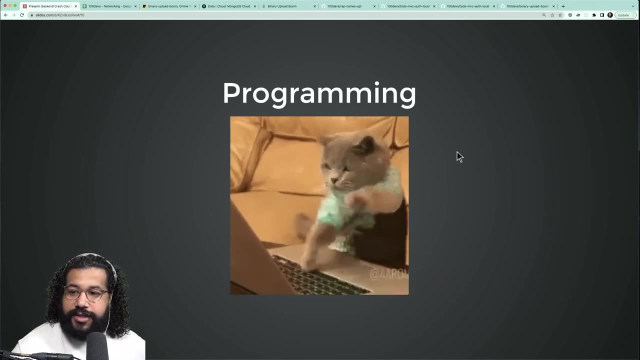 Do we store stuff into the database? Do we process credit cards, Do we log folks in? All this stuff that happens on the server and then figures out how to respond. Are we sending code, Are we sending JSON or anything back? Wonderful. So today we'll be talking mainly about the backend. 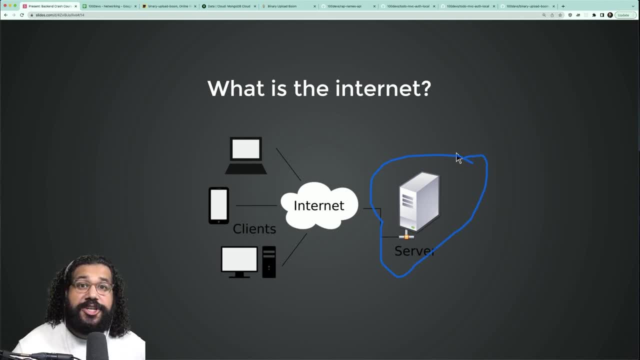 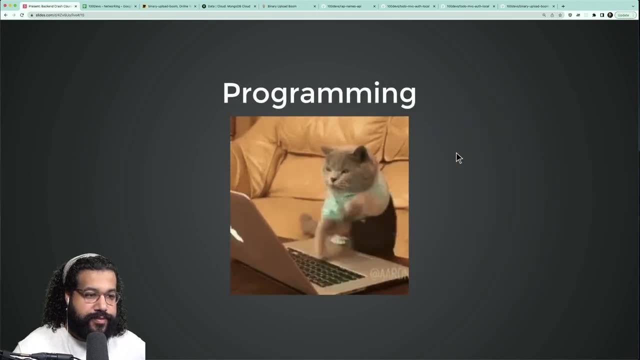 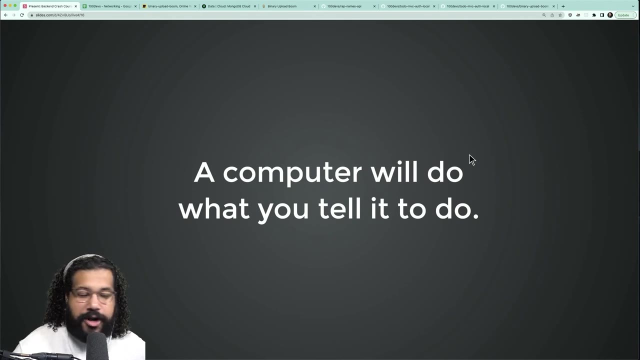 the stuff that runs on the server, That's listening for requests, That's generating responses, That's doing the heavy lifting to build out our applications. All right, Programming. As we talk about programming, we have to keep something in mind: A computer will do what you tell it to do, right, A computer will do what 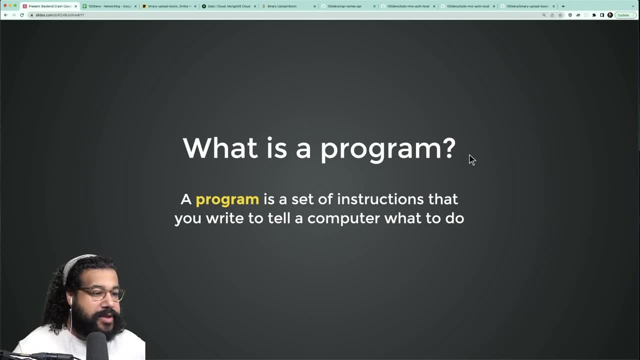 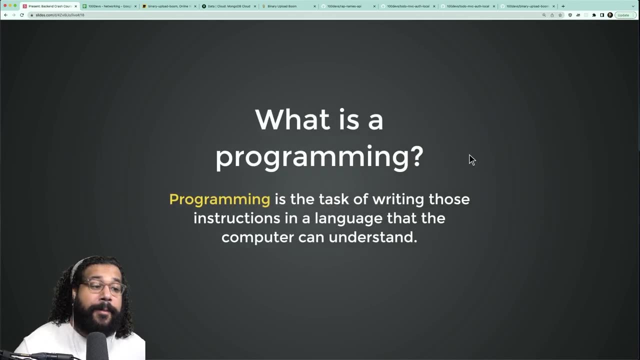 you tell it to do So. a program is simply a set of instructions that you write to tell a computer what to do, And that means that you're going to tell a computer what to do, And that means that makes the act of programming just simply the task of writing those instructions in a language that 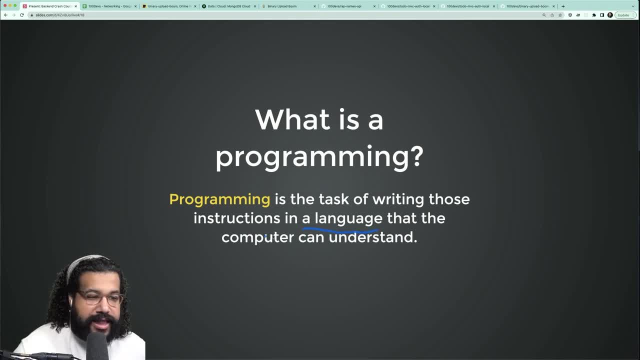 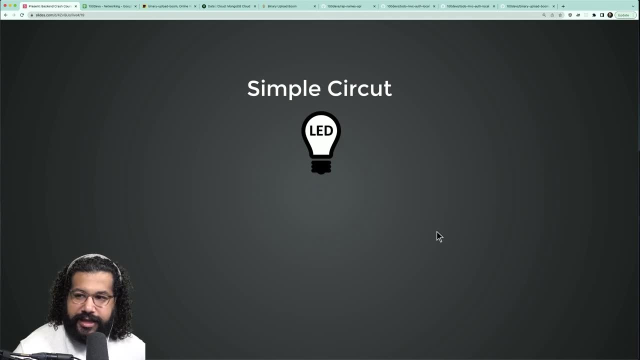 the computer can understand, And that's the important bit- the language that a computer can understand. So if we talk about this in terms of building up to a language that the computer can understand, I like to start with a simple circuit. Okay, Once again I got to grab my iPad. I don't. 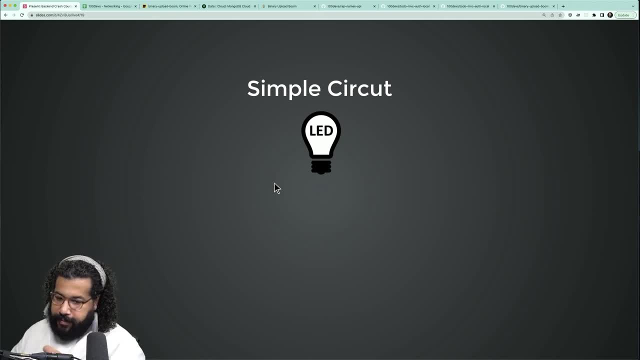 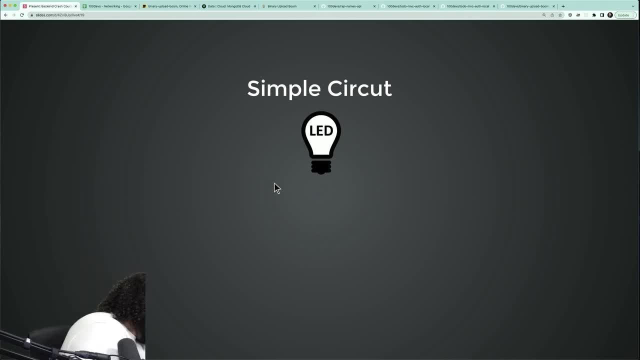 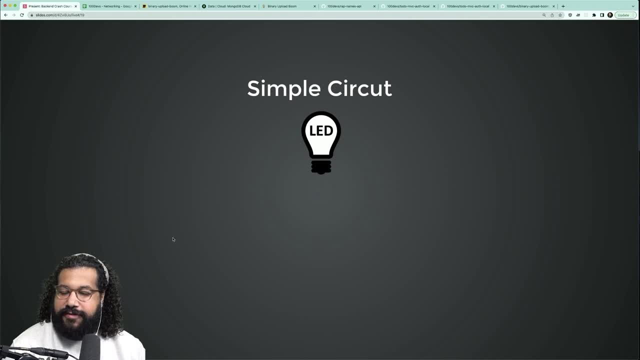 something to live for, a sense of pride and financial freedom. take care of your family: more pizza money so the family can get their best life. buy more digital goods on meta, not be on disability. help my mom go dead end job travel the world health care- i love it. thank you for sharing. so i don't understand why we're. 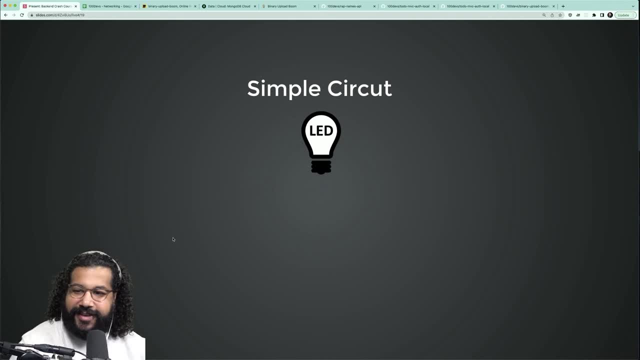 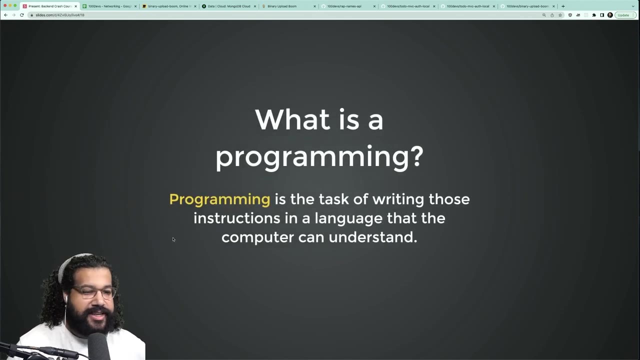 spamming wise, because you're all a bunch of nerds. i'm a nerd too, so that's okay. everybody starts typing the letter y in chat already. thank you for sharing that. all right, ipads, thank you. so programming is a task of writing instructions in a language that the computer can understand, so let's build up to that language. so. 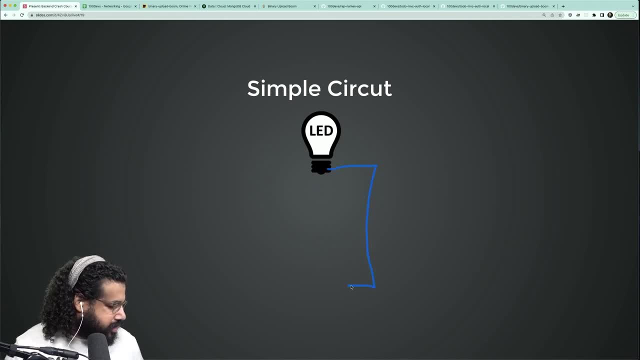 here i have a simple circuit, so i have my light bulb and i can connect a battery and since this circuit is complete- right, since the circuit is complete- the light bulb should turn on right a all right, so let's go ahead and introduce a switch into this circuit. so right now, 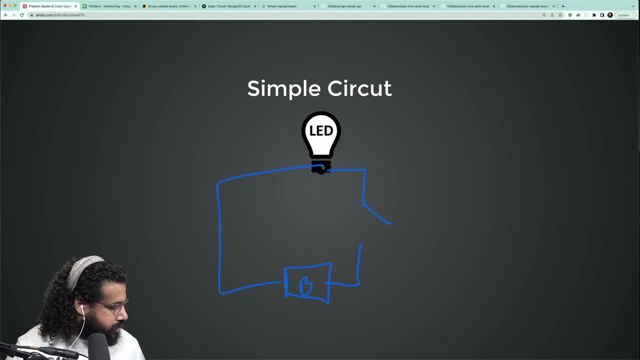 the switch is open and since it is open, is the light bulb on? nope, not on, and if I was to close the switch, the light bulb would turn on, and so we can represent this on off value with some very simple notation, right, so we'll say: 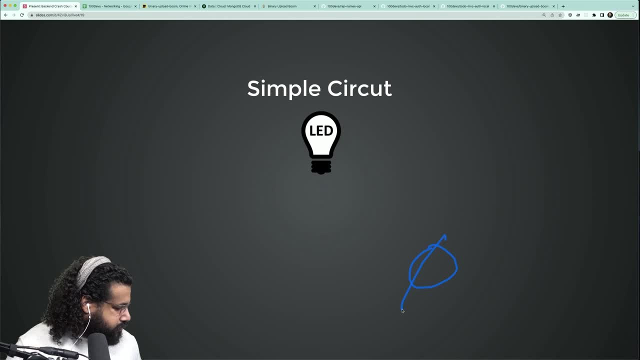 off is zero and on is one right, and so if i was to draw this circuit that had two switches, how could i represent this, this circuit? yeah, i can represent it as zero, zero or off, off. and how could i represent this circuit here, now that both switches are closed? how could i represent that? 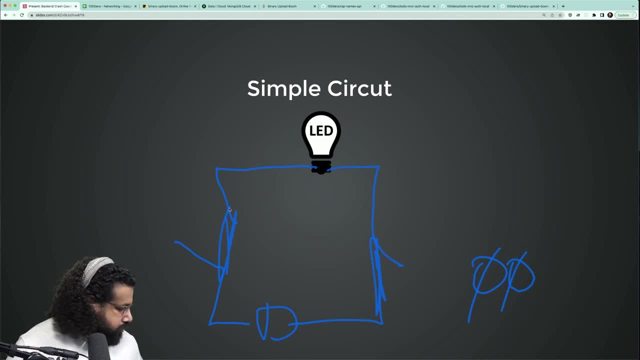 yeah, i could represent that as one one, right, one one, and so that means that i've now represented a circuit where both switches were open. i represented a circuit where both switches were closed, closed. right, we could also do. right, we could also do some other things like zero one one, zero right. 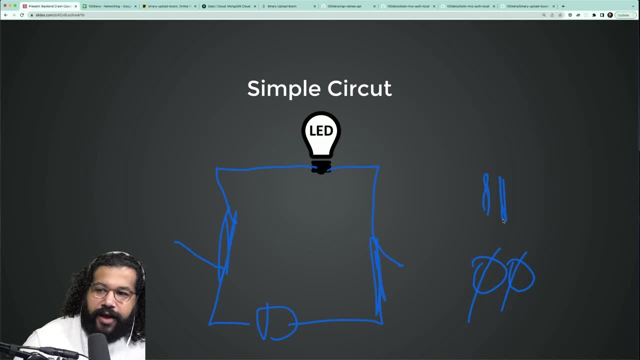 we could represent these very simple on off values in a very simple language, which we call binary. now, from this we can actually start to build up to a little bit of logic. booleans are c and g, or sugar that reduce to zero one. i love that. um, i actually can introduce a little bit of logic. 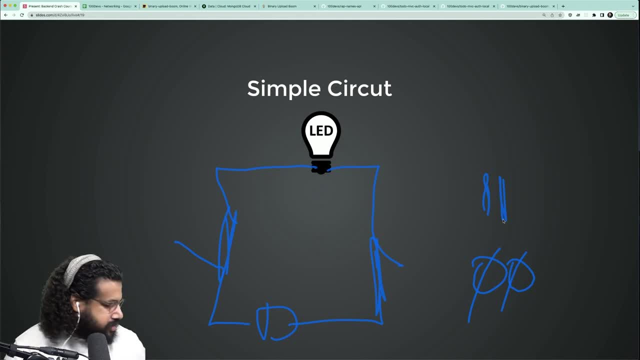 with the this notation. so, since both of these circuits are closed and i'm representing it with 1: 1, what would 1: 1 actually represent right now? like if we were to say: i think it's very simple, this is very high level. this is not meant to be exactly what's happening, but we can just think. 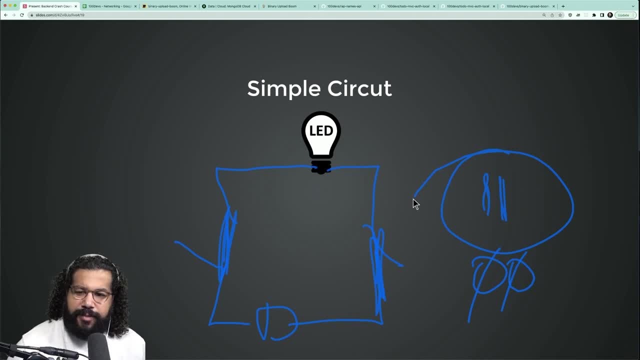 about something: yes, it's on, but we're talking about the inverse of what's happening. and then we could do like this, something which is like on 0, 1, and then we could say something like 2, 1, so talking about both of these switches, and we're representing that they are both on. so we would 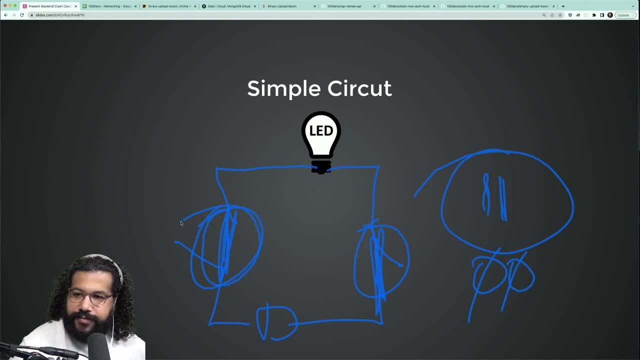 say this blank, this: yeah, and right and right. we're saying this one is closed and this one is closed, and so we can represent both right one one, and we can say that that means and like this one and that one, and so we can actually build up some very, very simple logic. right, we eventually call. 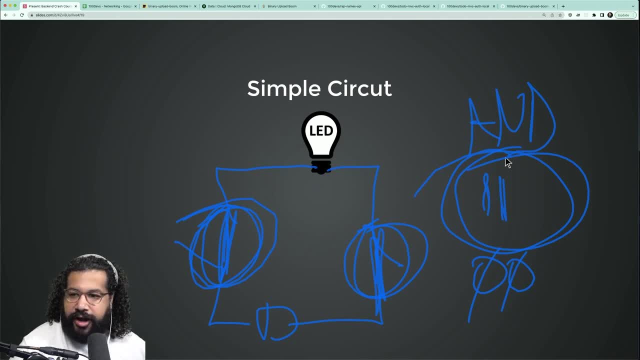 these things called logic gates, and just by representing on and off values and adding slightly more gates that are on and off, we wind up with things like and nor like all this other fun stuff that you'll see when you kind of nerd out about this stuff. but the idea here is that 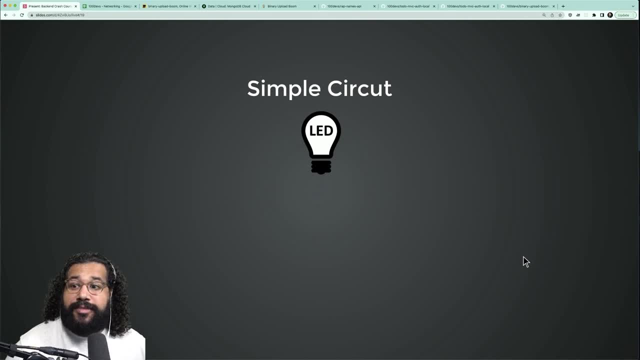 from just simple on and off values, we can build up to some logic. we already saw and right. all right, we already saw and and we can start to utilize right. once we have simple logic, we can then build up a very low level programming language once we add things like memory. 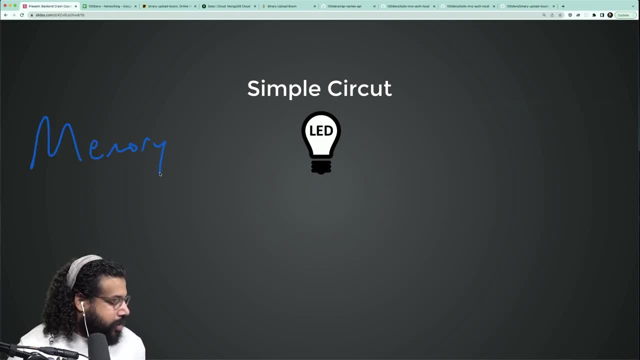 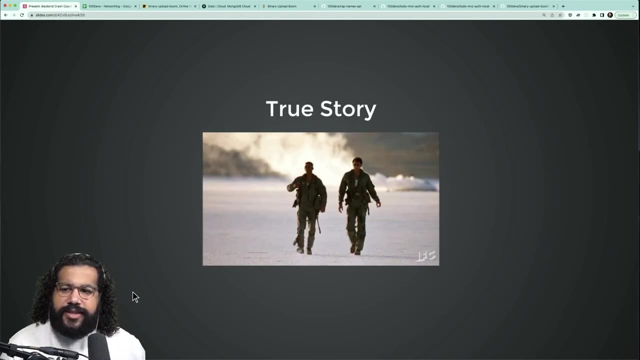 right, a a way of doing some a basic arithmetic, and we have some very low level logic. right, we can build out a programming language. however, the language that we're we're learning is still very, very simple. right, so we can build up a very low level programming language and we can build out. 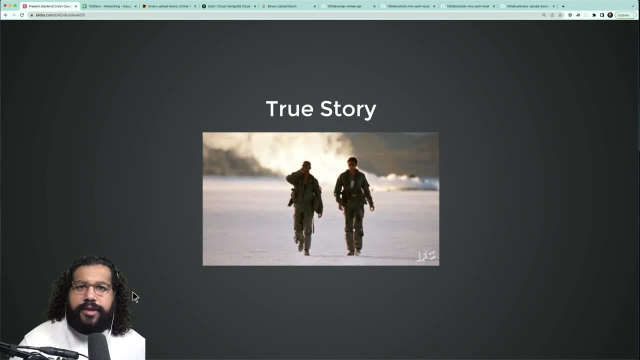 a very. that would be very, very low level for us. we're not going to be writing this low level like assembly level code on a day-to-day basis. i'm going to be writing something that is a little bit more human readable. and talking about human readable- uh, true story for those that don't. 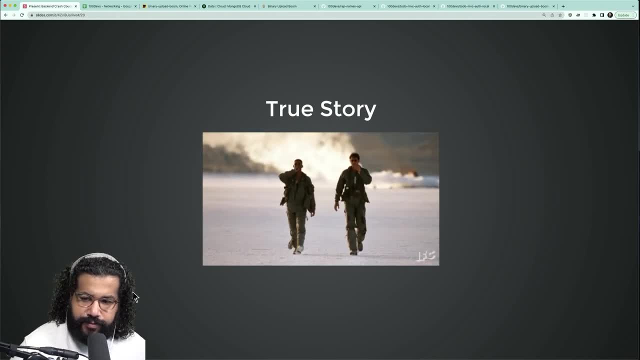 remember, uh, independence day, right, aliens came to attack the world and we were able to destroy them. now, if you remember, when the aliens first came, uh, we tried to nuke them, we tried to do all these wonderful things and uh, we couldn't. we couldn't do anything. they had these wonderful force shields. 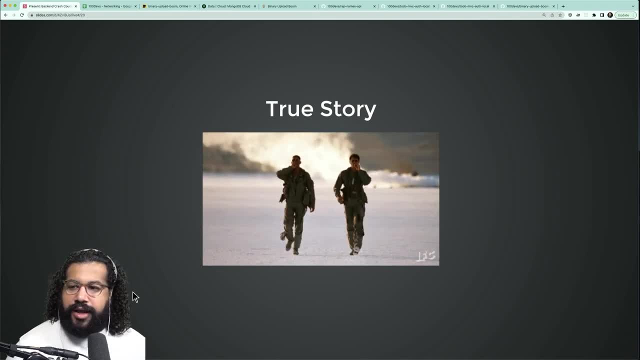 but what we did realize is that we had one of their, one of their previous planes that had crash landed years before and when the alien mothership got close, that spaceship got power. so there's something about that. that's what we're trying to do right now. we're trying to do something. 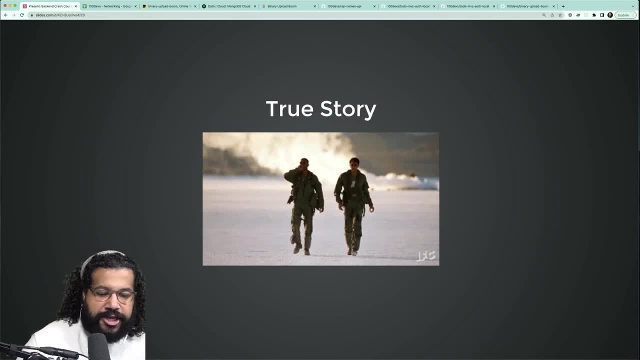 about how power is distributed across these alien ships, um, something about how the force field comes on when it's near other alien ships. and so there's this idea that if we could like turn off power on the mothership, maybe that would distribute to all the other ships and, uh, bring their force fields. 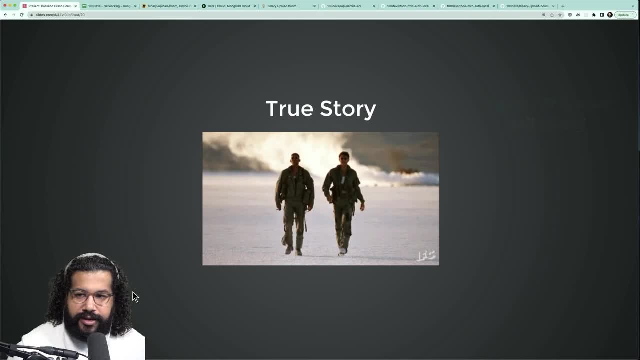 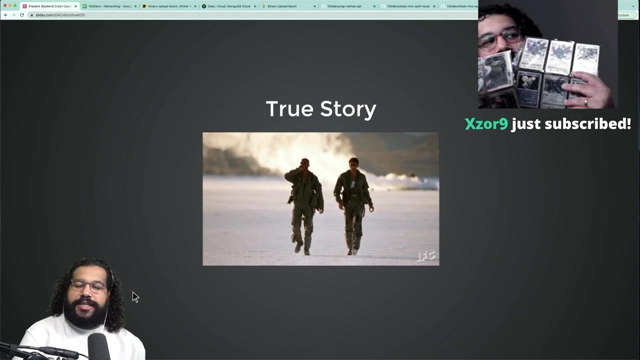 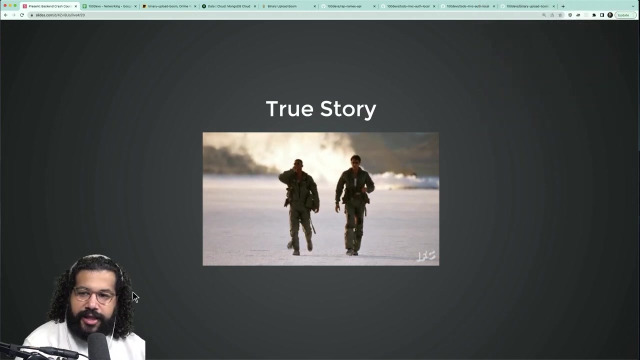 down so that we could, uh, you know, nuke them and and save the world. so what did jeff goldblum do to save the world? yeah, he wrote a computer virus that they then uploaded to the alien mothership. that took down uh, the the power, or distributed uh, the power, uh, to these other ships force field. 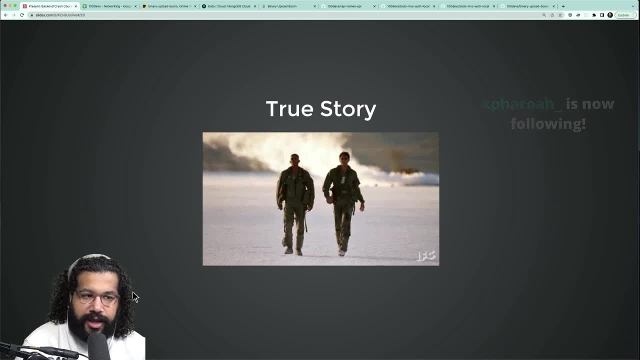 turned off and we were able to blow them out of the out of the sky. uh, how in the world did they do something like that? one conversation with a group on the preparation for the technology: um, uh, um. however, the yeah, jeff glow and uh had a. 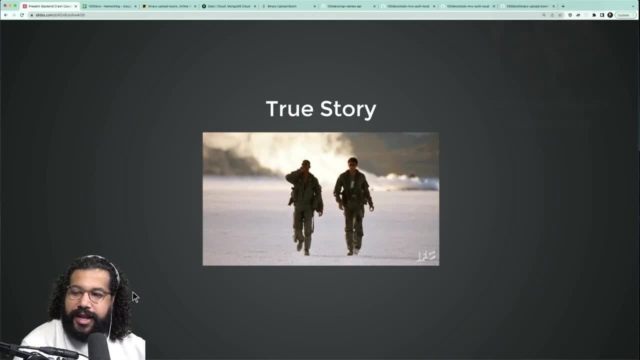 lot to do with um, yes, yes, um, on zeros and ones, the on and off values. We would assume that on and off is a universal constant. So this idea of building up to more and more complex logic would be the same, no matter if you're here on earth. 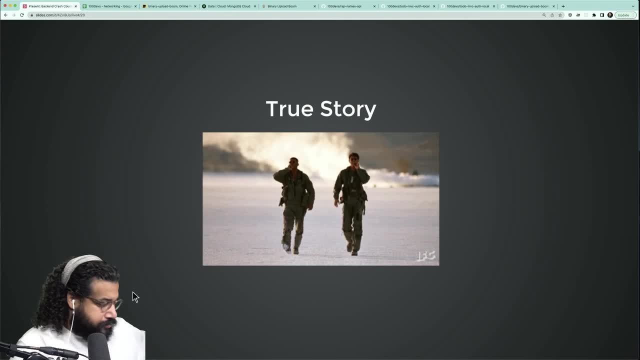 or you're aliens far, far, far away. So Jeff Goldblum reverse engineered their language all the way down to zeros and ones and then built it all the way back up into a language that they could inject into the alien mothership. 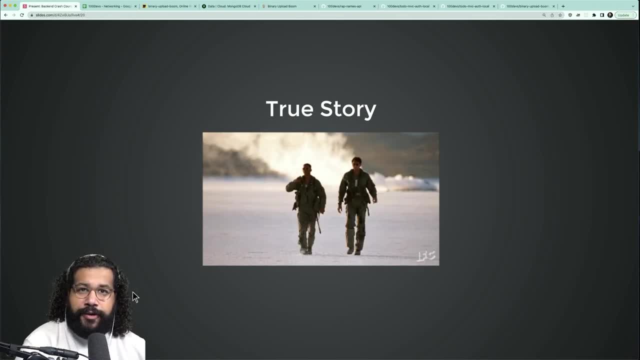 We refer to this wonderful event in history as binary upload boom. We took down all the ships and Jeff Goldblum saved the world, America right National hero. And so this is a true story right, And this idea is that we could theoretically do this. because, at a very, very low level, all the languages that we are writing can be broken down into on and off values, zeros and ones built up to more complex logic, more complex logic. But us, as programmers, on the day-to-day, don't wanna have to worry about writing binary. 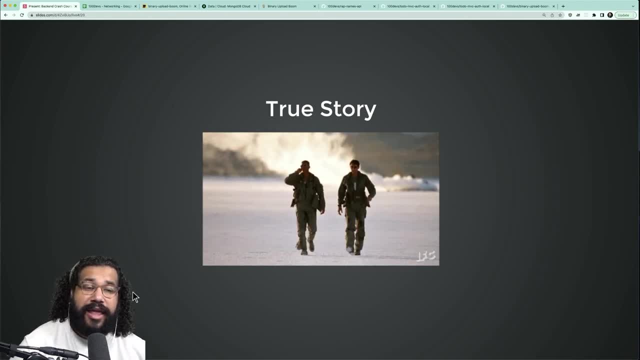 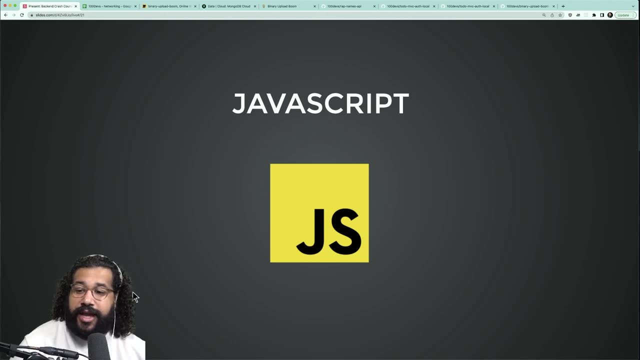 writing assembly level code. We wanna be using something that makes our lives easier, And that's JavaScript. JavaScript is the language that we're using so that we can work well together as engineers. We can communicate our complex ideas and then, underneath the hood, right. 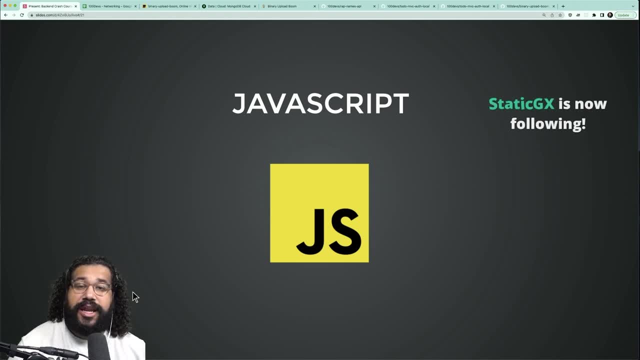 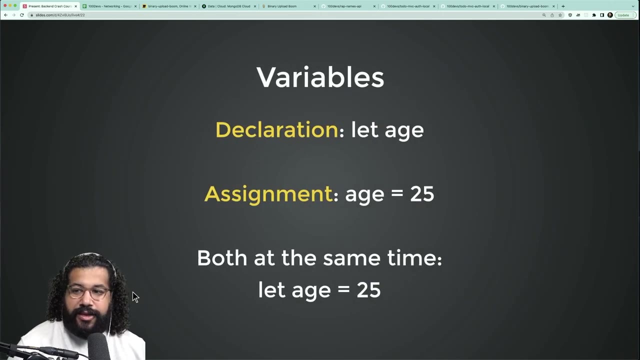 Underneath the hood, this JavaScript is getting broken down into that simpler logic that our computers can understand, But it's not something we have to ever worry about, because JavaScript is doing the heavy lifting for us. Cool, Now some basics, just to get them out the way. 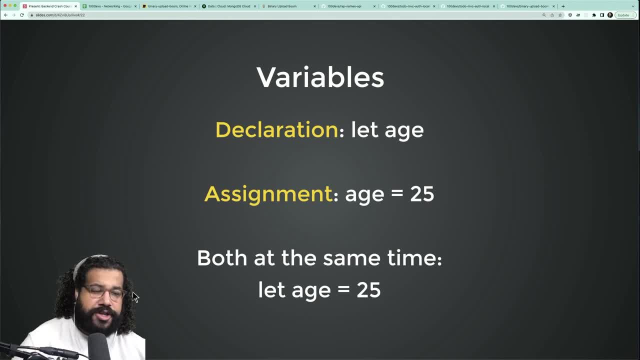 especially for folks that are kind of really new. just that we're all on the same page as we get deeper into the review. And don't worry, we're gonna go through this kind of quickly and we'll jump into the more meaty stuff pretty soon. 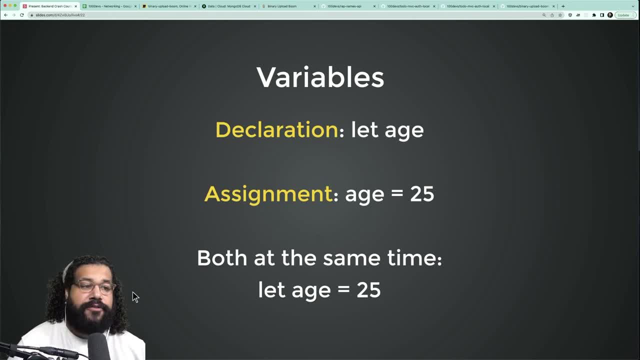 And also just to clarify a quick caveat again, uh, for those that are new or kind of uh, jumping ahead a little bit with the catch-up crew, today there's a lot of stuff that we go through don't feel like this is the class or the moment where you have to learn it or fully understand it. this is meant to be a review, uh, for. 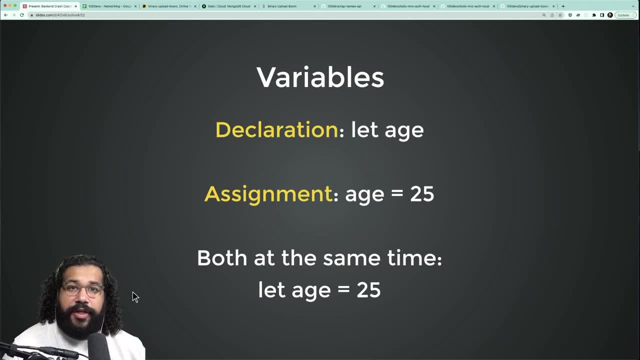 folks that have been kind of watching along and so know that there is a class for each and every single bit of information that we're covering today. feel free to jump on discord to ask questions. feel free to ask questions here in chat. i ask everyone that you answer questions that you 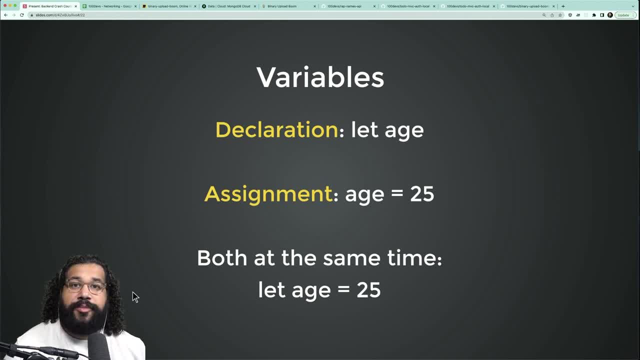 see in chat and then, um know that you can always go back and watch individual classes to shore up a lot of this material. all right, uh, variables, uh, so variables, uh, enable us to store information. so we have this idea of when we talk about kind of computing, we have a space in memory. 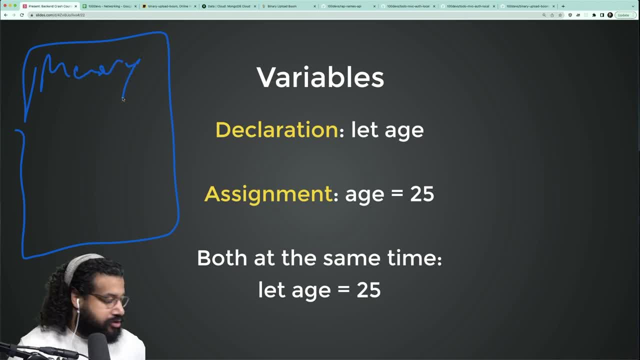 you and our variables enable us to create that space in memory with a step called declaration. so i would create a space in memory called age and then i can assign that space in memory of value. so then i would put 25 in that space in memory. so i can do this declaration creating. 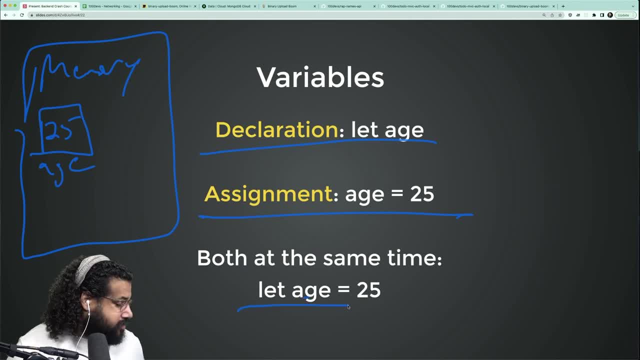 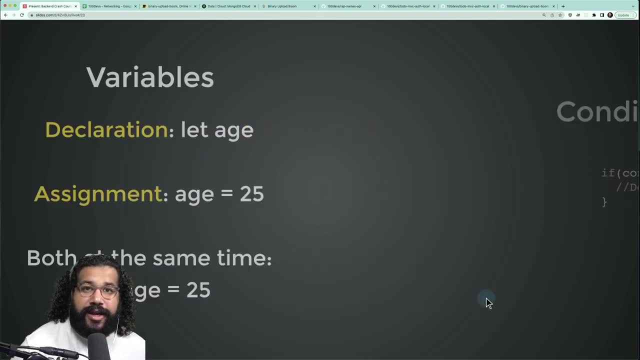 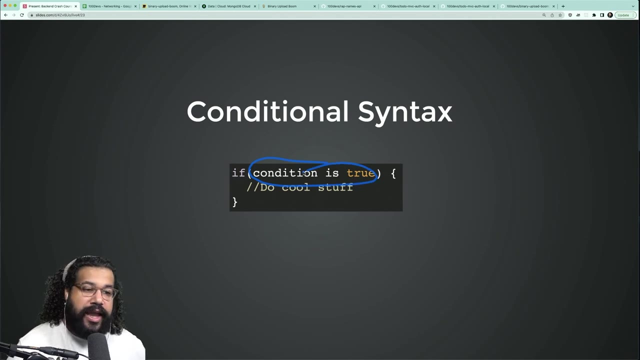 the space in memory and assignment on the same step. so here you can see: let age equal 25, i have declared my variable and assigned it a value. at the same time, boom, we also have a space in memory and also set a secondary value as well. so it creates a. 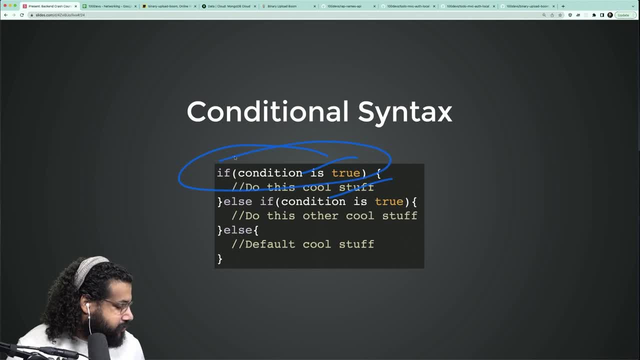 set a template here where we can do that on the inside of the brain. we can also have conditional syntax where we can check to see if a statement is true, and if it's true we wind up doing what is inside of the curly braces. 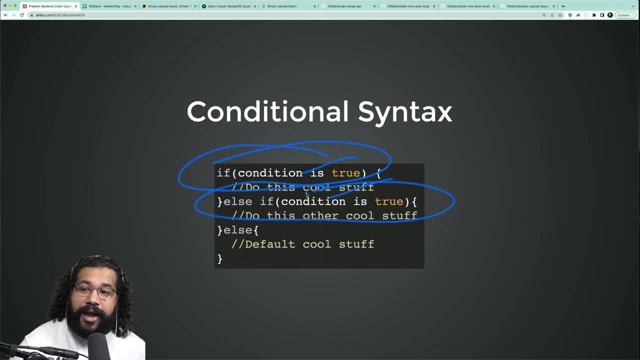 ifs are true, the else will auto magically run right. the else will automatically run rfn 972. so where can i find the previous videos? you can do exclamation point youtube here in chat to find our youtube, but don't just watch on youtube. also join our discord, exclamation point. 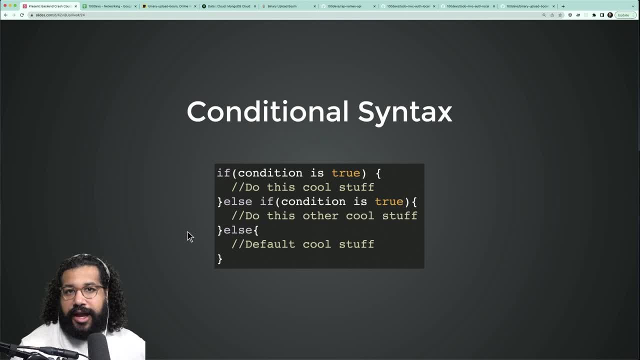 discord. that's where you'll find all the materials and you'll find our community. where are we at now? let's see, that's wild. that's just wild to me, that's absolutely wild to me. we are at 39 589 people. 39 589 people on discord. that's wild. 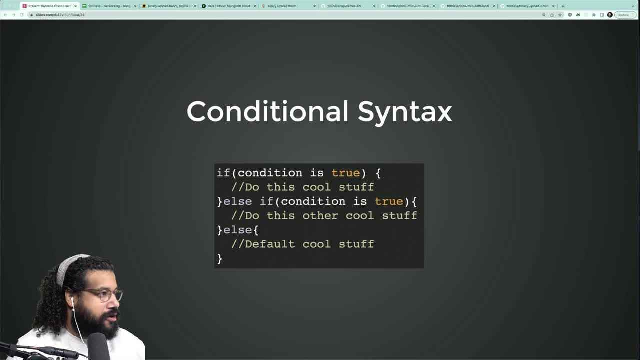 how many bots, uh, we have. we have like four or five bots that run on the channel, but, uh, we are like our like everything's dialed up to the max, like it's. it's, um, you have to do like phone verification and all that stuff um, but the cool thing is you can actually like see, 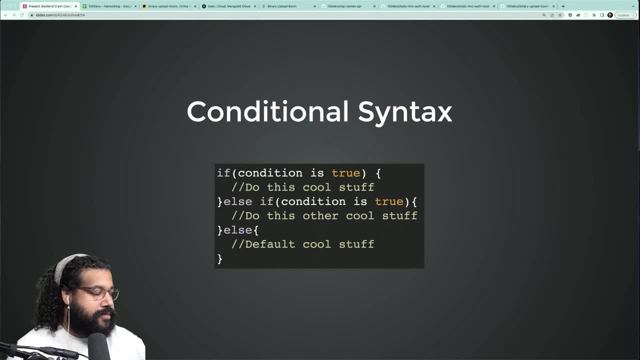 um, you can actually see um the number of active folks and at like any given time, there's like 4 000 like actively online. that's bonkers. that's wild. yeah, that's wild cool, uh. so here is a lovely bit of uh syntax. here we have conch pizza equals dominoes. uh, why is? why is this pizza const? 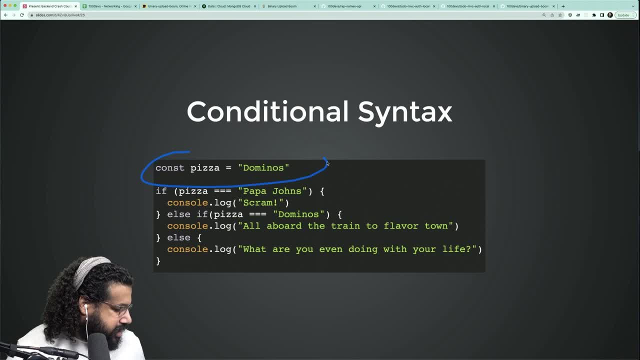 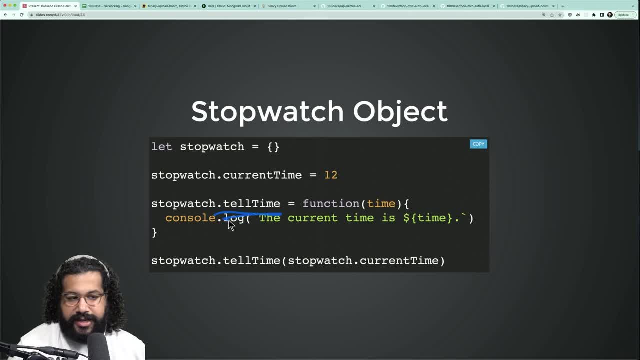 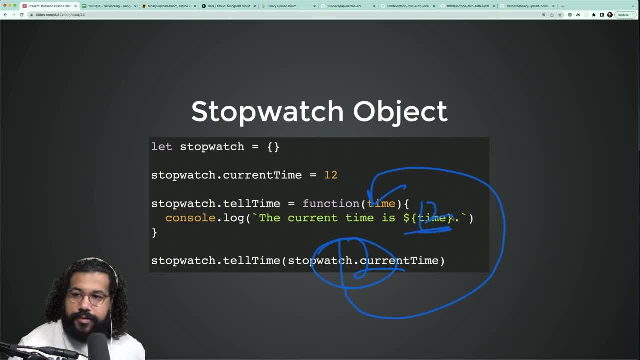 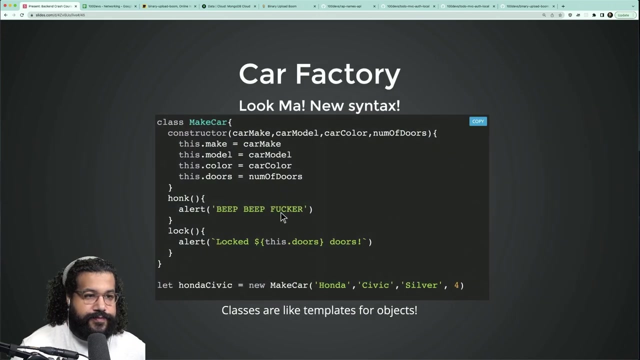 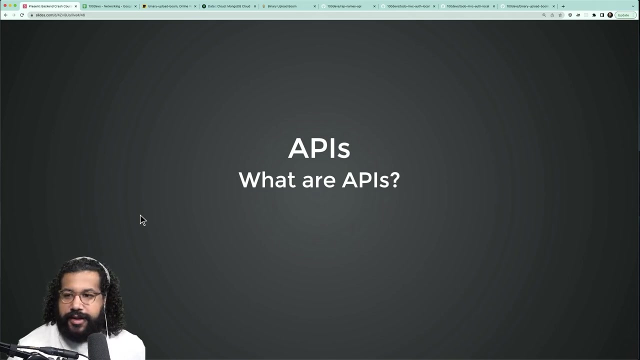 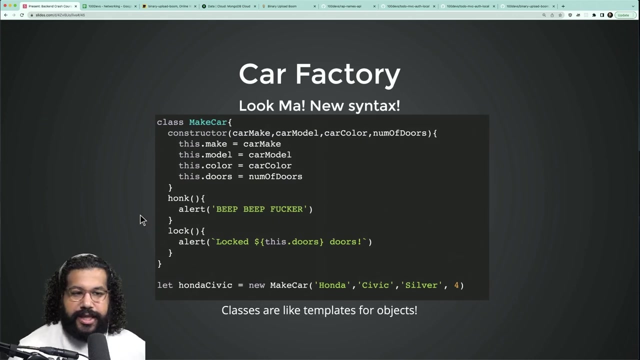 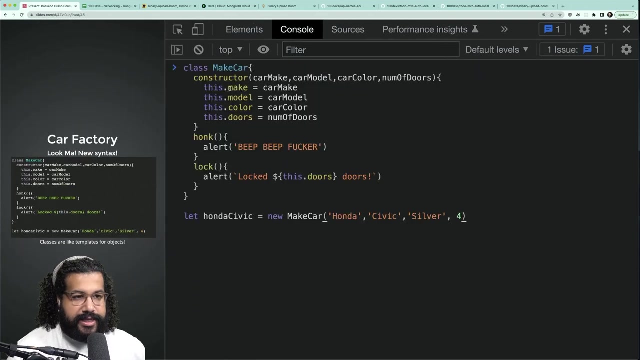 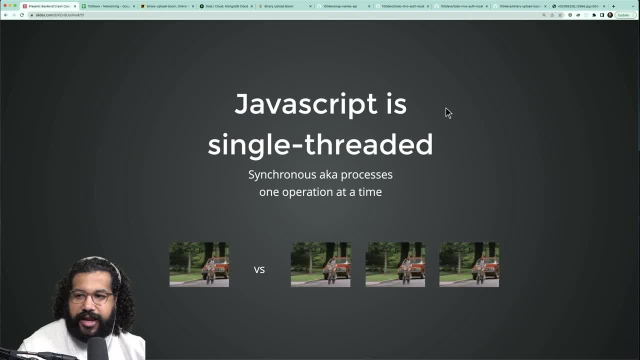 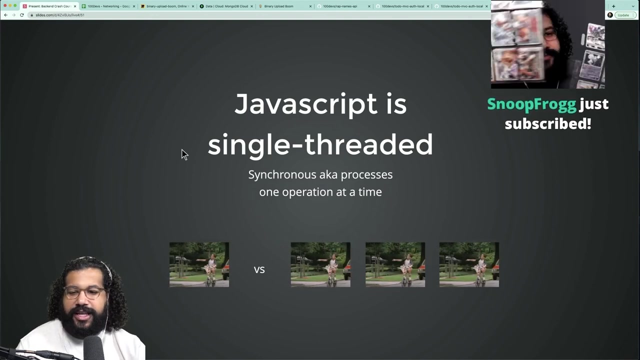 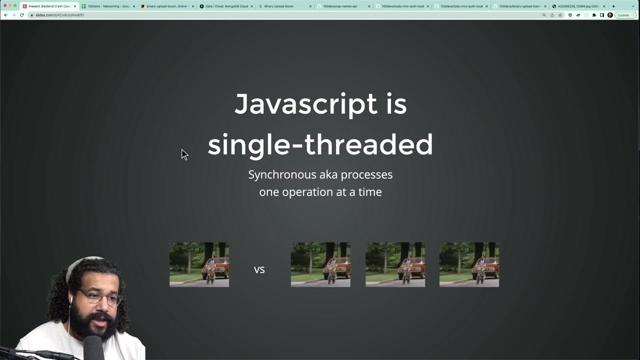 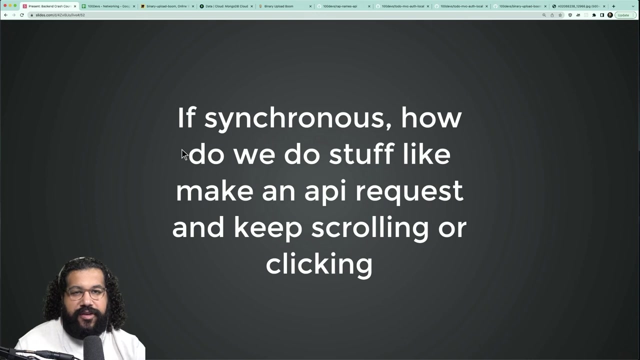